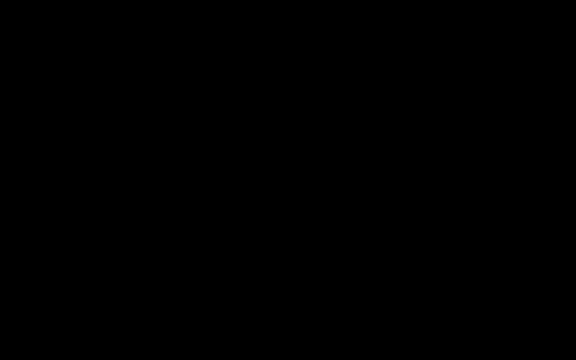 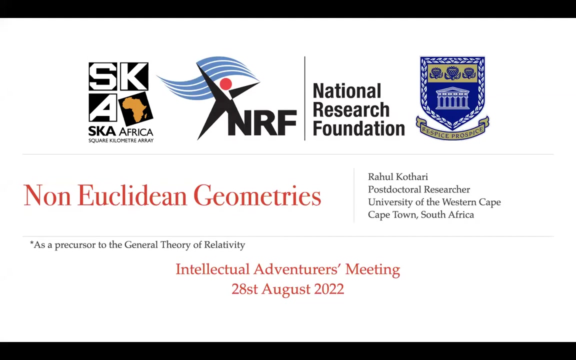 This video is about non-Euclidean geometries, So let us begin then. I welcome all intellectual adventurers to this meeting. Today I will talk about non-Euclidean geometries, So this will be a precursor to perhaps a future talk on general theory of relativity. 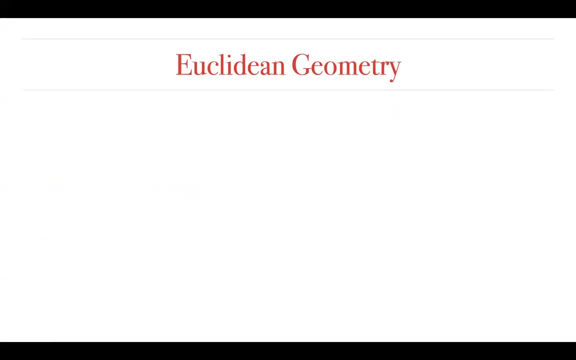 So first, before talking about non-Euclidean geometries, is my voice audible? Yeah, your voice is clear. Okay, So before talking about non-Euclidean geometries, let us first talk about what is Euclidean geometry or geometry in general. 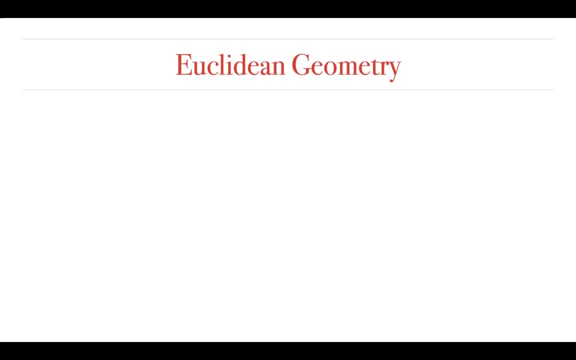 Because geometry and Euclidean geometry are kind of synonymous, Because Euclid is so famous because of his book Elements. So this is the guy, Euclid, who wrote a book called Elements, And Elements is considered to be one of the most read books in history. 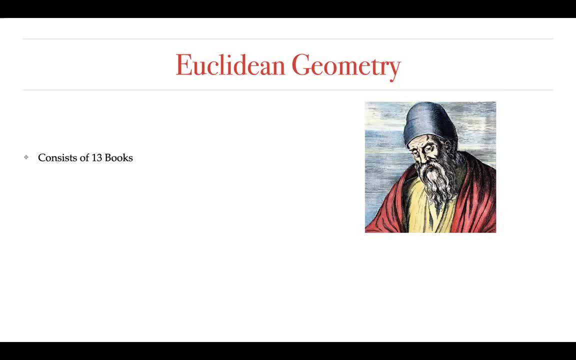 So perhaps after Bible, this is the most read book in history. So this contains of 13 books. So the first book starts with a lot of propositions or results related to geometry, Circles, triangles, etc. etc. So first book also has definitions. 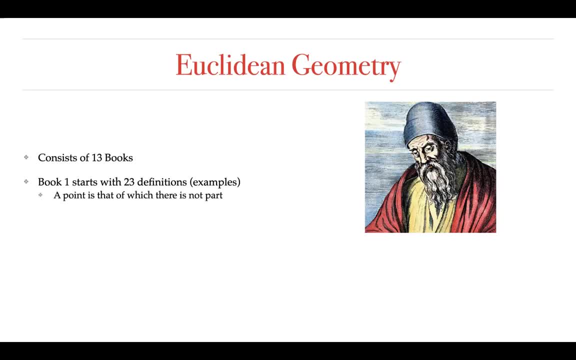 For example, it says that a point is something which doesn't have any part, Or, in simpler words, it doesn't have any dimension. And another thing is: a line is a length without breadth. I mean some kind of common notions, Some kind of very intuitive things. 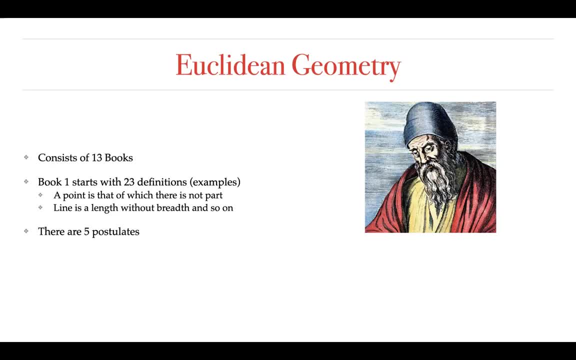 And apart from these, there are five assumptions, postulates, or axioms As we call them these days. So just a second. Gyanthi was calling me. Okay, Just a second. Will it also pause recording? I don't know. 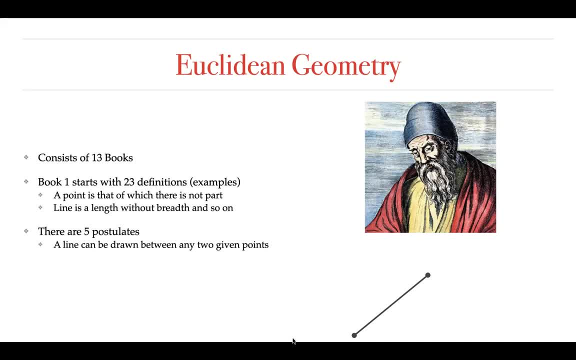 Okay, So will it pause recording? I think it will. Okay, So I'm going to play it again And I'm going to make sure I have the right key, So I'm just going to play it again. I'm going to play it again. 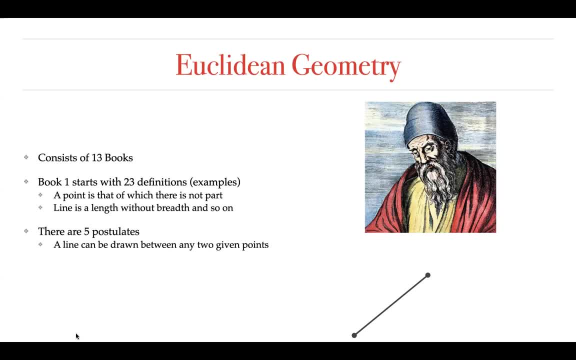 Oh, here it goes. So I'm going to play it again. So I'm going to play it again. Here it goes, I'm going to play it again, And the next thing is okay. so, as I was saying, there are five postulates. So one of the postulates: 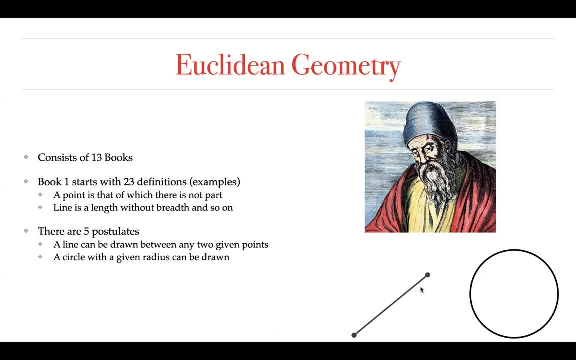 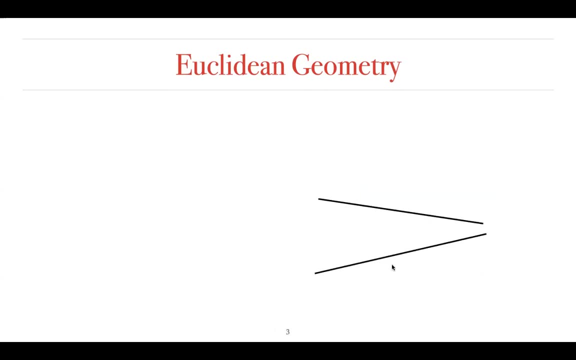 is that a line can be drawn between n to given points. Let's say, this is A, this is B. you can always draw a line between these points, And this is an assumption okay. And given a circle with radius something, let's say C and radius R, you can always draw a circle. 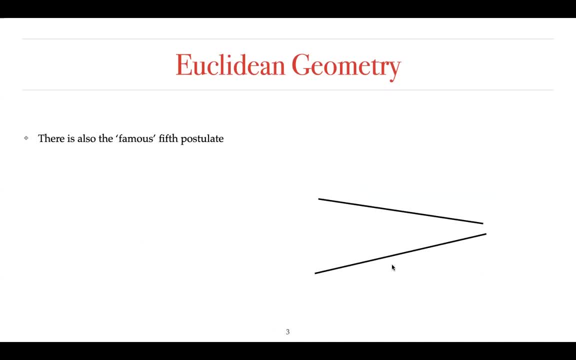 Okay, But apart from this, there is also the famous fifth postulate. I said it famous because of the reasons that will follow now. It says that if you have a straight, let's say if you have two straight lines and there is one more straight line that is intersecting these two straight line, at these. 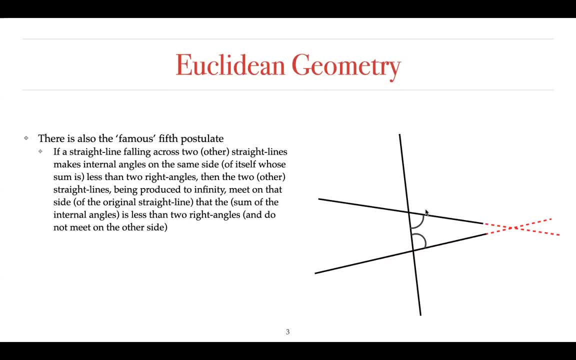 points. let's say m and n, and on one side, let's say on this side, if the sum of the angles is less than 180 degrees, then if you extend these lines further, they have to intersect at one point. So this is the famous fifth postulate, And it created a lot of confusion. 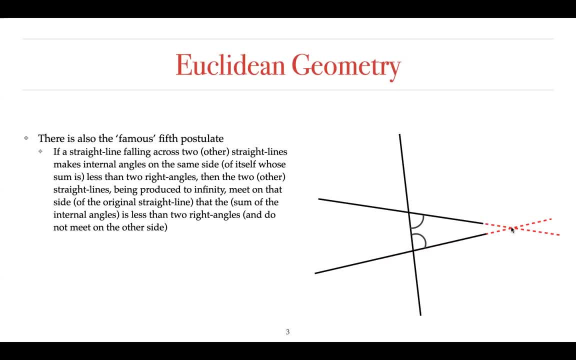 as well as motivation in the community of mathematicians generally speaking. So the thing was how to, or is it possible that you can prove this axiom or the postulate with the help of first four? But okay, so this is the story that I'll talk in the forthcoming 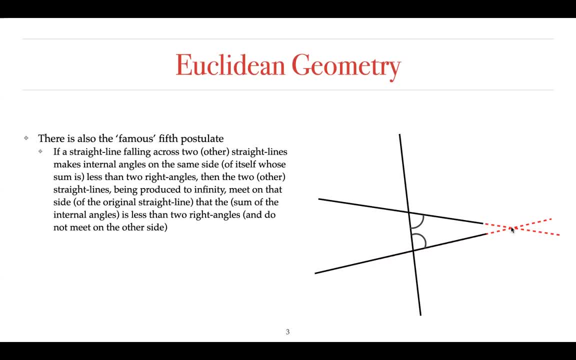 slides, But for the time being, I mean, this turned out to be a very, very important postulate. So, apart from this, there are some common notions as well. So, for example, one common notion is: if you have so, this says that if you have A equal to B, you can draw a circle. 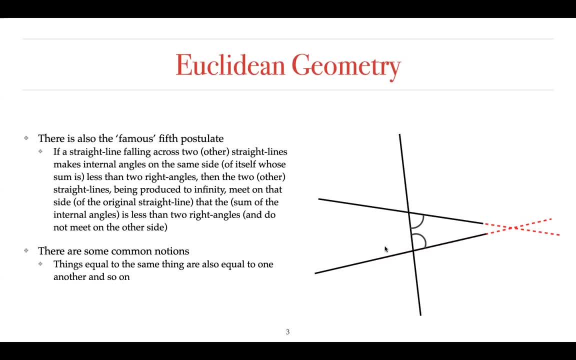 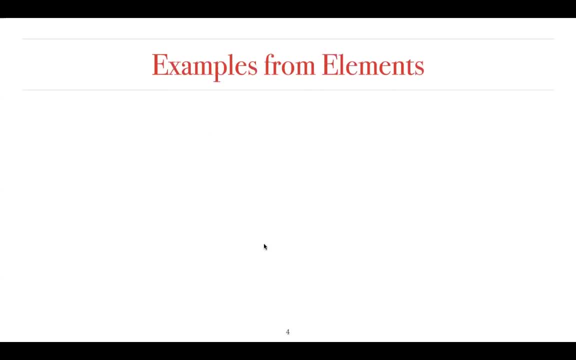 And for B equal to C, then it follows that A is equal to C. Okay, So, okay. So now let me take some examples from the elements. So elements is a vast book consisting of so many propositions, theorems, corollaries, etc. So I mean, so let me talk. 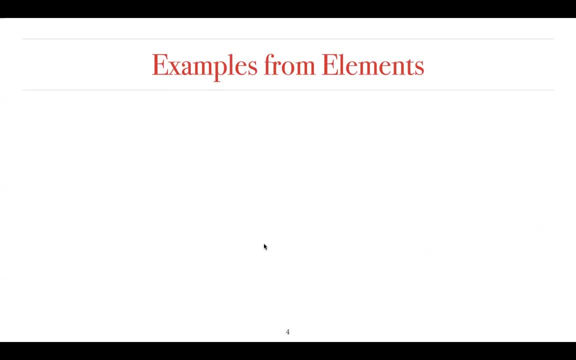 some of them now in order to appreciate what kind of reasoning it involved, what kind of simple reasoning and so elegant reasoning it involved. We can draw more detailed videos out of this stuff, But let me bring it closer to what exactly the general sense and what we each do as mathematics and other materials is. So another 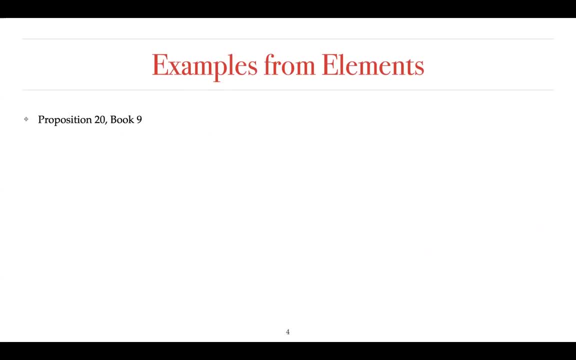 thing it touches us is that I think it is quite Right offhand very good, tricky right You involved. so i'll take a proposition from book 9 and and, and that is proposition number 20.. so proposition 20 of book 9 is about the prime numbers, that there are many, many infinite number. 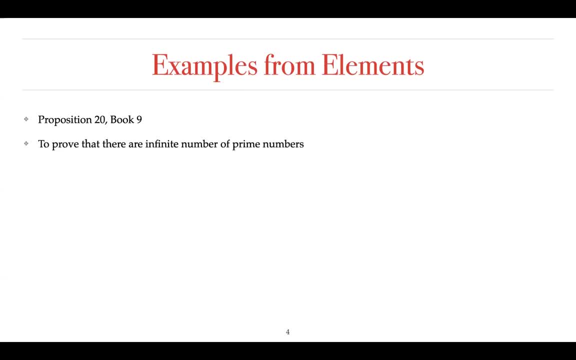 of prime numbers. so, and the proof goes in this way: so, nikhil, am i audible? still audible? yes, sir, you are audible. yeah, okay, okay, fine, okay, so, so now we. so now we want to prove that there are infinite number of prime numbers. so, so this is how the proof goes. so so we use it, uh, by using: 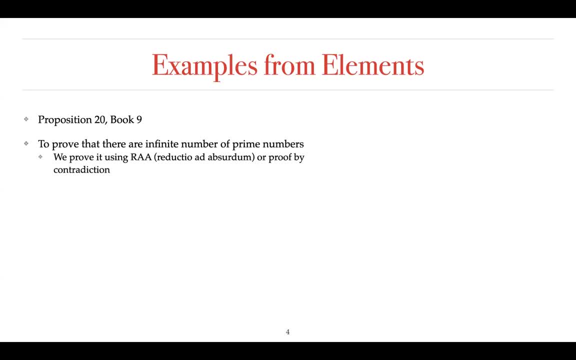 something called as reductio ad absurdum or, in common language, proof by contradiction. so so this is a very, very famous and and favorite rule of mathematicians. so so they use it quite often. so they use this uh tool called the reduction absurdum quite often. so this is how the proof goes. 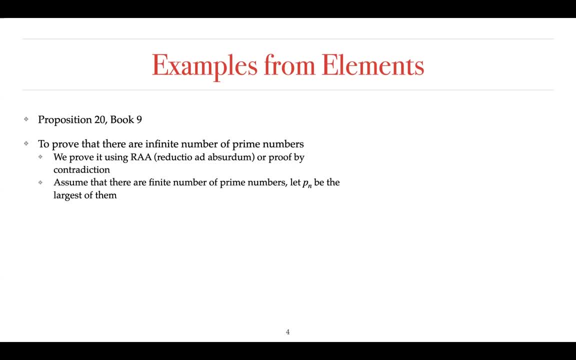 so let us assume that there are finite number of prime numbers. so if there are finite number of prime numbers and let pn be the largest of them, because they are finite number, so there has to be some largest prime number. okay, and now you make a number which: 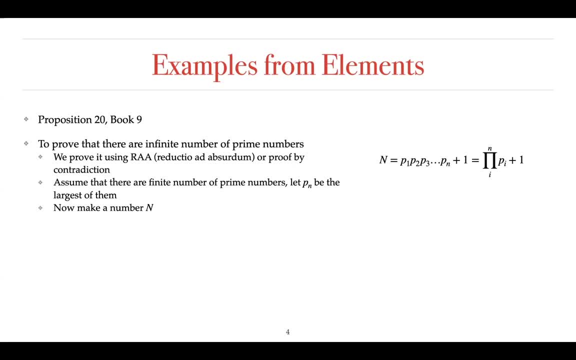 is equal to the product of all these, all the prime numbers, is smaller than pn, and you add one to them. so this is what you do. so p1, p2, p3 and pn was the largest prime number, and you multiply all these prime numbers and add one to them and you get another number, n. so now what happens? so now there. 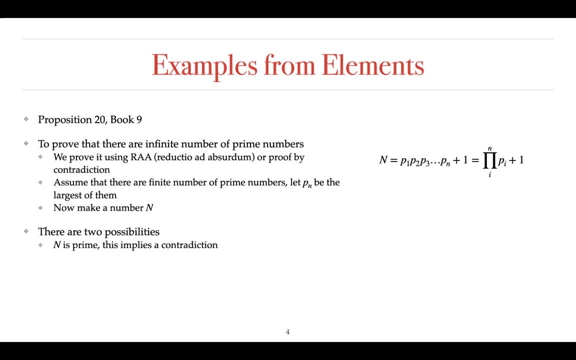 is this number n, so either. this number is a prime. so, for example, if you take the largest- i mean this is only an example- if you take p and to be two, so and you, and if you do this, you will get three, three is a prime, very good. so, and two into three plus one is also a prime. 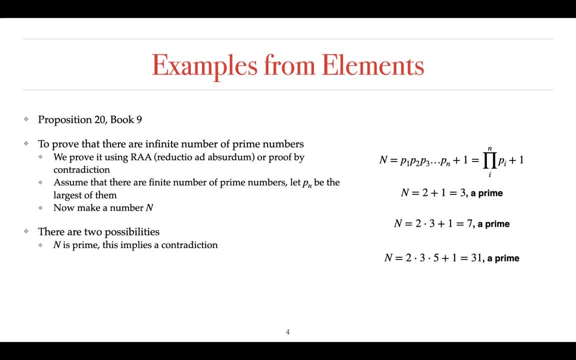 two into three, into five, plus one equal to 31 is also prime. so you get a contradiction, because because you said that this is the largest prime that you will have, but by doing this you are getting even larger primes. so so this is a contradiction. so, if so, since this is leading to, 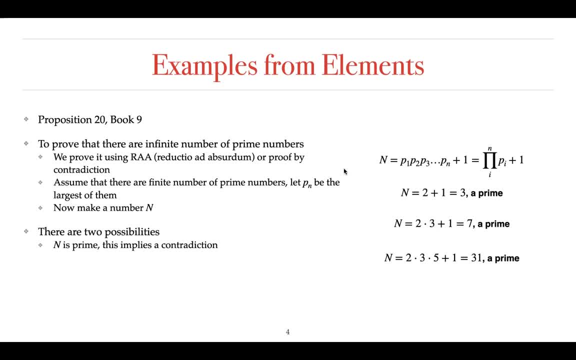 a contradiction. your original assumption must be wrong. so this is how it is done, but there is one more possibility. so one more possibility is that the number you get after doing this multiplication is not trying, so, for example, in this case: oh sorry, i'm sorry, i forgot to put plus one here. 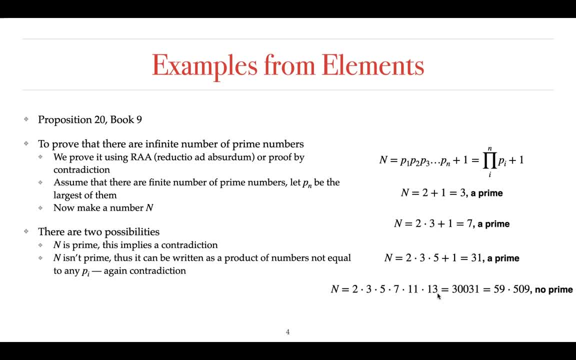 okay. so if you do this and if you add plus one to it, you will get three zero zero three one, but which is not prime and which is equal to the product of 59 cross five zero nine. but this number is larger than this. so, because if a number is not prime, it should. 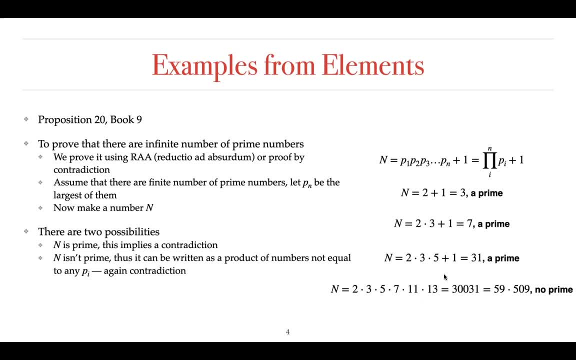 be written as a product of two primes, or at least two primes. so either this is a prime or this is not a prime. so if this is a prime, then it is a contradiction, and if it is not a prime, you can write it as a product of other primes which were not there in the list before. 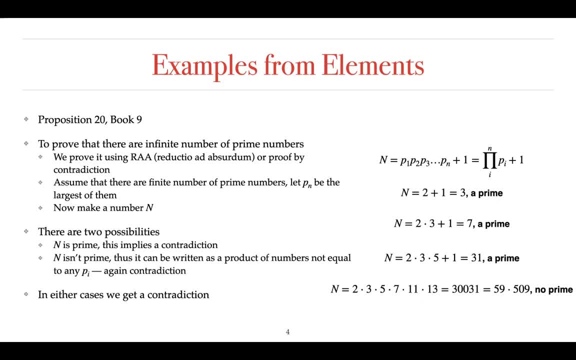 so in either of the cases you get a contradiction. so thus there has to be an infinite number of prime numbers. is this good enough? is this okay, okay? good so, okay, so. so this is one example from the euclid, uh, from the, from the euclid's elements, and, and there are, and there are so many, i mean. 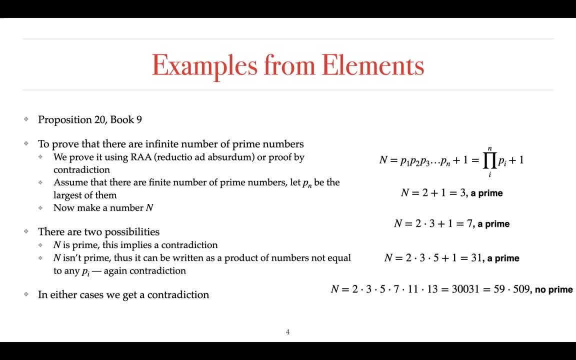 uh, it's literally very, extremely beautiful book to read. it's an extremely beautiful book to read. i mean, i have not read it completely, but but whatever, some of the chapters, do you have the hard copy? uh, at one point of time i had, but now, uh, actually, when i left iitk, i left. 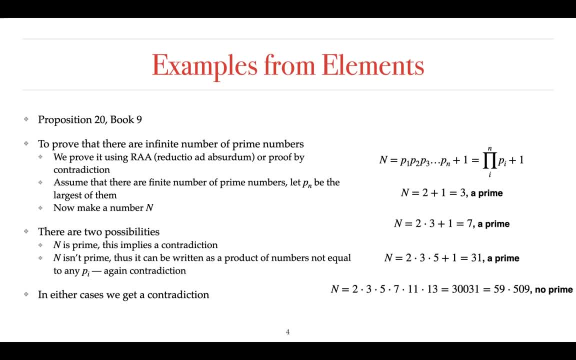 all those books there i do. this is uh, this is uh equal element. yeah, yeah, from from the elements, yes, from the element. so so this is proposition 20 of book number nine. yes, yes, yes. so this is perhaps i. i just want to add one line suggested. so every, every reading scientist used to admire this book. 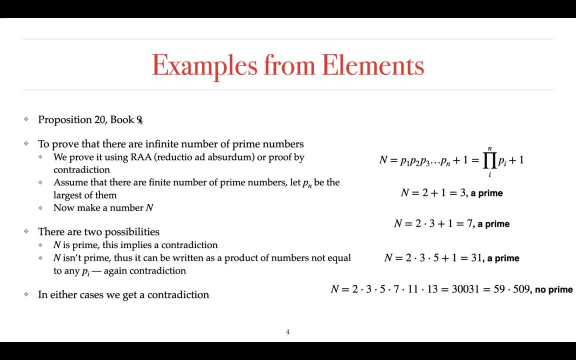 so even i understand. once i said, if at all i have to go to an isolated place for a long time, i will go with euclid instead of either element. yeah, it is. it is extremely beautiful book to read. i mean, it is so satisfying. honestly, it is so satisfying. 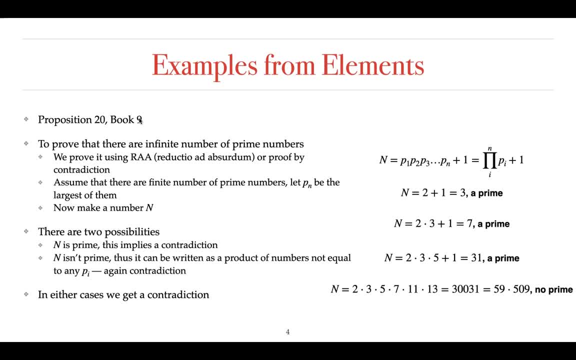 yeah, it's a foundation of home. yeah, it, it, it all. it is also kind of foundation of the modern mathematics, because modern mathematics works in, works along this direction, so in modern mathematics. so so, whichever field you choose. so earlier they did not have axiomatized the probability theory, but kolmogorov finally. 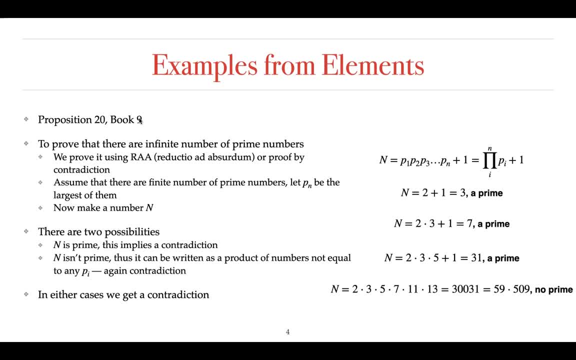 did that. so that is also an axiomatic theory. so now we have axiomatic theory of probability, and analysis is based upon nine field axioms, and so on. and linear vector spaces are also based upon nine axioms. and finally, and also arithmetic. arithmetic is 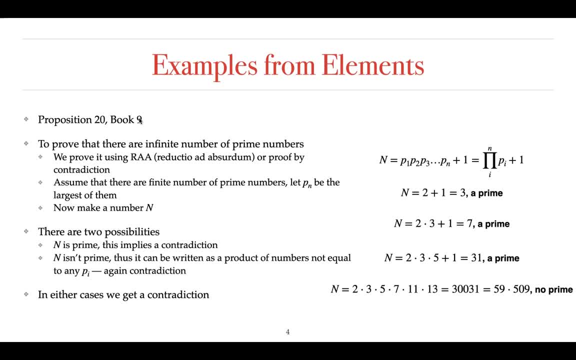 based upon piano's axioms and so on. so so they have taken i mean um. so in the, in that sense, the modern mathematics um is kind of based upon what euclid did about 300, not 300, but 2000, okay, so yet another example from the euclid is this: 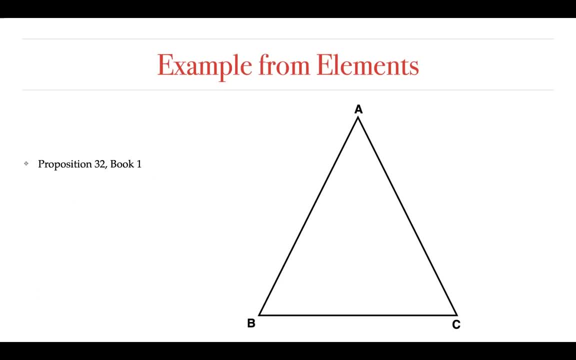 so. so that is proposition 32 of book one, and i i know this is very familiar to you because you must have seen this also. so so this says that let a, b, c be any triangle, as i've shown here. so if you uh extend one of the sides, let's say you extend this side and let's say this angle. 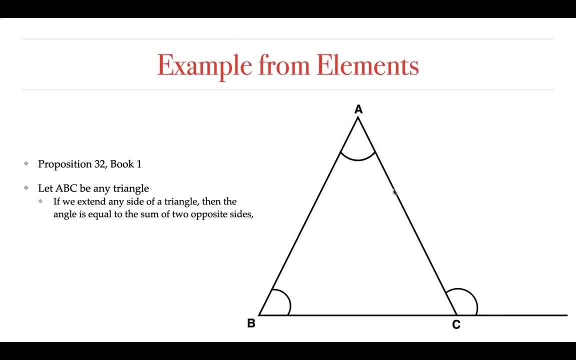 is a, c and something. okay, i should have put here d. so if this angle is acd, then this is equal to the sum of opposite angles. so this is equal to the angle sum of this and this. so this is one part. sorry, were you saying something? no, sir, maybe some voice from my side, i will mute. 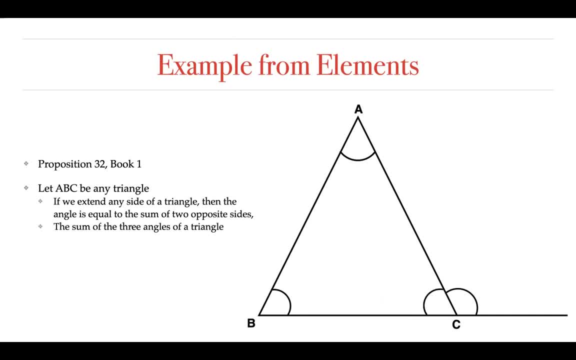 okay, okay so. and the other, and the other part of the state and the other part of it says that if you add all three angles, angle a, angle b and angle c, you will get um is you, you will get 180 degrees. it will be equal to this. it will be equal to 180 degrees. oh, i forgot to put it here anyway, but but. 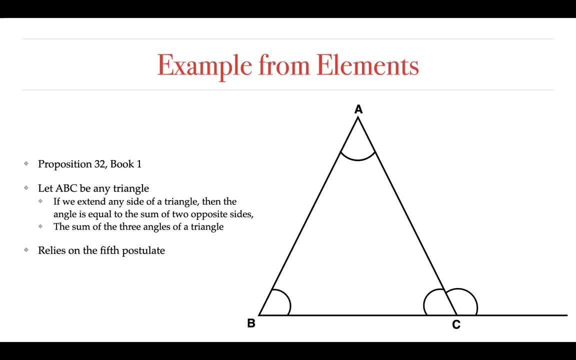 let's put that this one, both sides of the angle have their own angles and they have their own angles. and we now relies on the fifth postulate that we discussed, uh, some time ago, okay, and uh, so. so this was the original fifth postulate- that if you have two lines and you have another line, that 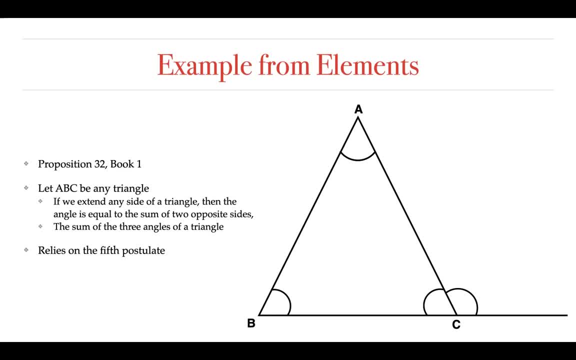 intersects these two lines. and and uh, if the sum of the angles on either side of the line that that was intersecting is less than 180 degrees, then if you extend the lines they will intersect that side where the sum of the angles was less than 180 degrees. 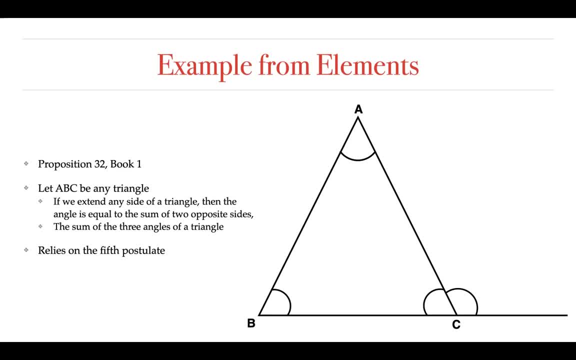 so. so one is called as the play fair axiom after the mathematician play fair. so play fair axiom is perhaps- uh, i mean- easier to grasp or easier to say in words. so so what it says, if we have a straight line, let's say any straight line and a point that is not on the straight line. 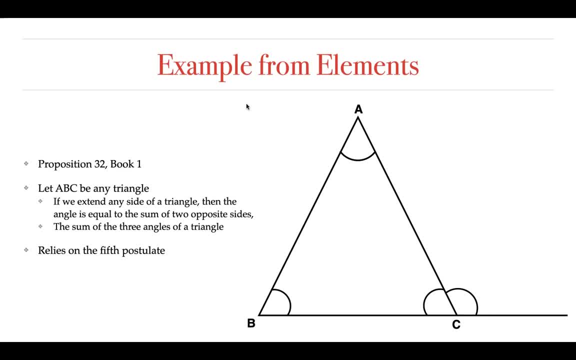 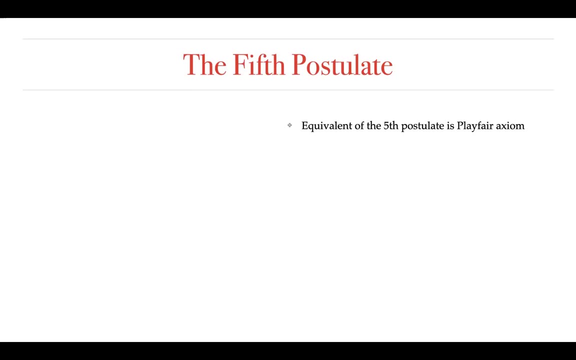 you can draw one, and only one straight line that passes through that point. okay, i'll show it next. okay, so let us, because fifth postulate is so important, let us talk a bit more about the fifth postulate. so, okay, so, as i just said, it is uh. so an equivalent statement of the fifth postulate is: 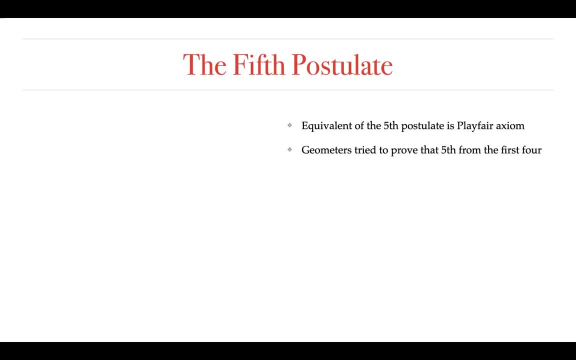 called a prefer axiom. so so geometers really tried hard to prove for the fifth postulate of the axiom from the first four, but they miserably um failed because it was not possible. they found that it was not possible and fifth postulate is a separate logical. 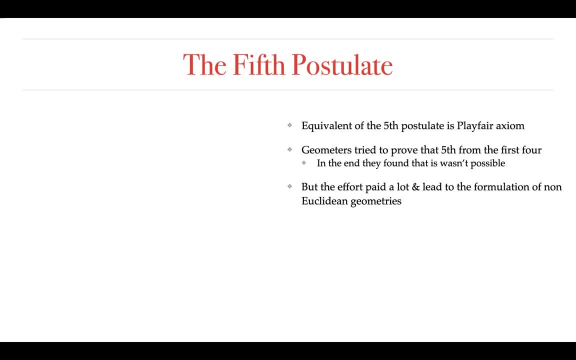 possibility, but they're stereotypes, so so it was not possible for them. but they really swiped and they actually took management of the first post and um moved the dedication of fourth postulate and so in particular Educationalist啊, and paintings árte sидENTра kinsperis, they réponse to this case. 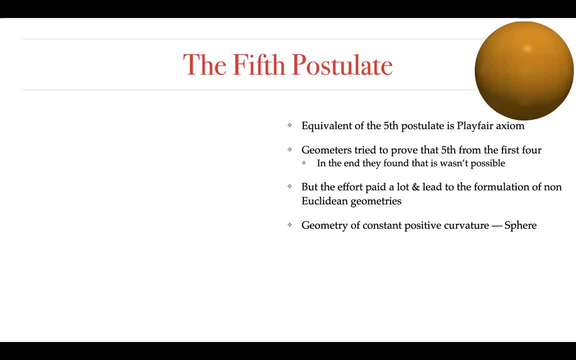 yeah, the number one view had experienced Racette factor, so mainly on the set of bursaries. but unfortunately most of this analysis didn't rasa bore any fruit. for a bystander of the of a well, yourself, pretty much all this material and, uh, for this example i'm going to think of what is the 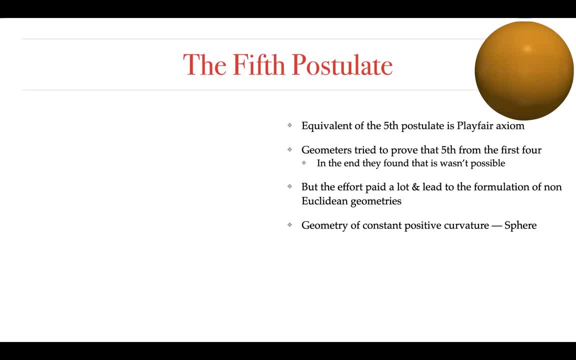 if i can say that, because in case of euclidean geometry, the sum of three angles of a triangle is always 180, but, as i will show in the next, in the forthcoming slides, it is not true in the case of, for example, sphere or other geometries that i will also speak about. so, but uh, so this example. 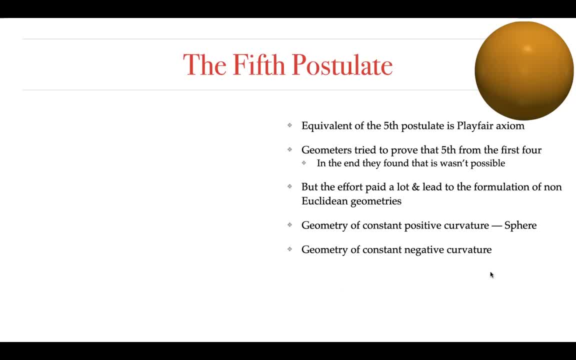 was known for a long time, but this took really some time in order to be discovered. so this was about 1850s or so, 1850s or 1860s. so three persons, uh, gauss, carl friedrich gauss, the great, the prince of mathematicians, carl friedrich gauss, uh, and janos boliai and lovachevsky. so these were. 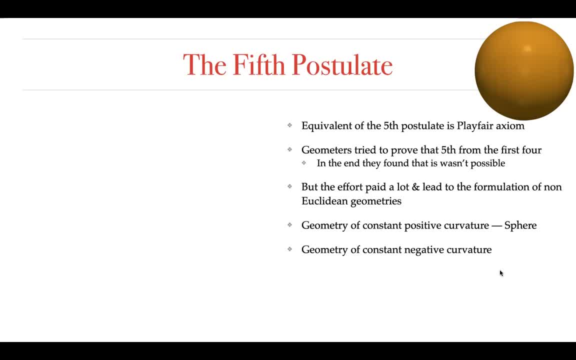 the three mathematicians. so, and they separately did that. so, so their, so their research was: let me put my okay, okay, am i still audible? yes, sir, okay now, now it's better, now it's being better, okay. so, and and and another example was surface of constant negative curvature. so one way of realizing, i mean so. so this is an example, or 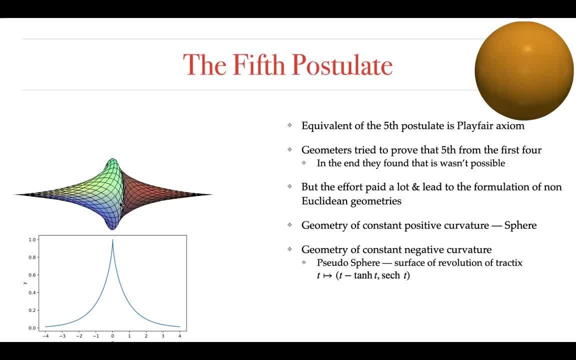 rather, um, okay, okay, okay, okay. So this is an example- or perhaps the only example that I am not sure about, but this is an example- of a surface which has constant negative curvature. So this was the case when you have constant positive curvature, but in this case you have constant negative curvature. So how do you? 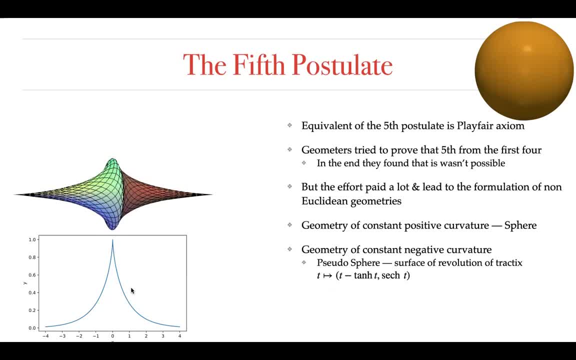 get this. So this is the parameterization of this curve. So this is x coordinate, this is the y coordinate. So if you plot it as you vary t, you will get this, And if you rotate it about the x-axis, you will get this. So, although- and one more thing is, although, it appears that it- 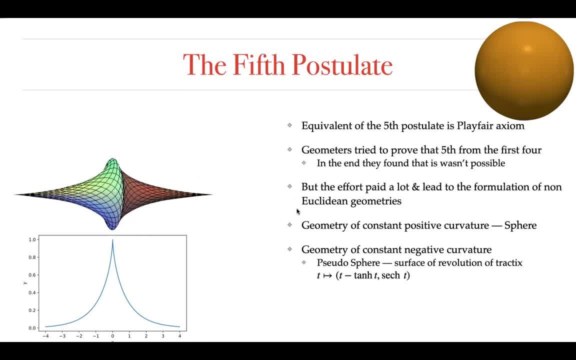 kind of terminates at this point, but this is not because this goes till infinity. This never ends. So these are not the terminal points And this continues till infinity. So, and these are the three persons as I was talking about, Karl Friedrich Gauss, Janos. 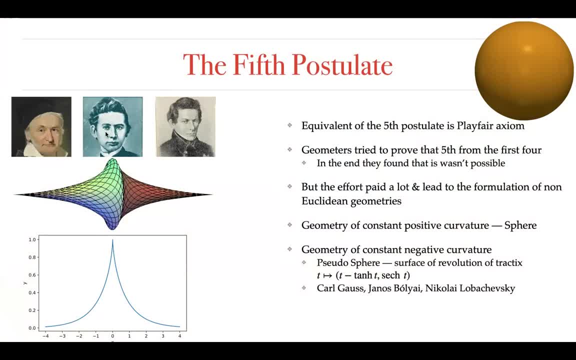 Bolli and Nikolai Lobchevski, So a German, Austrian and a Russian. So these persons individually. So these are the three persons individually, So these are the three persons independently discovered this example of constant negative curvature. I mean this, and it is. 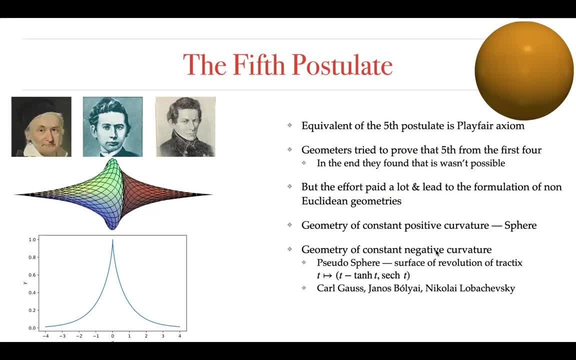 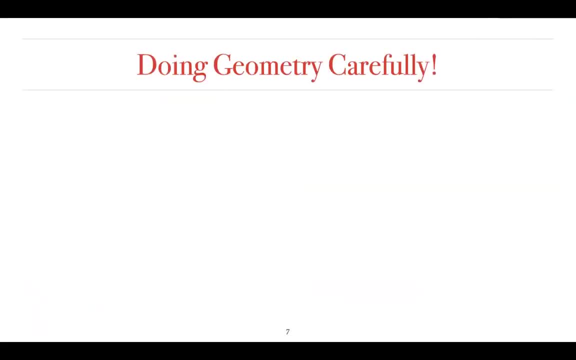 we also call it as a Schroeder sphere, because a sphere has a positive curvature. A Schroeder sphere has a negative curvature, So okay, So one thing is: I mean so now, since we know a bit about that, the fifth axiom does not hold, So we perhaps 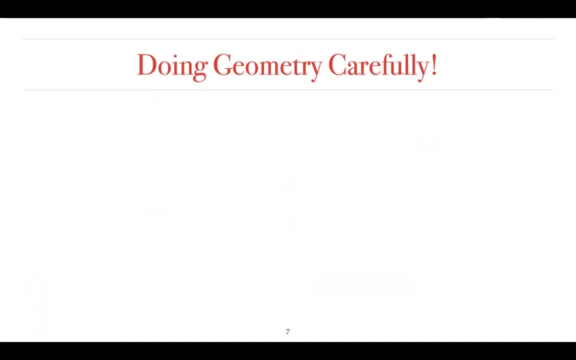 need to do our geometry a bit carefully. So why? by carefully? I mean so we have to have precise motions of straight lines, circles, etc. etc. So let us try to do it, the geometry, a bit more carefully by using, by relying on just the definition, Because if we rely on the definitions, 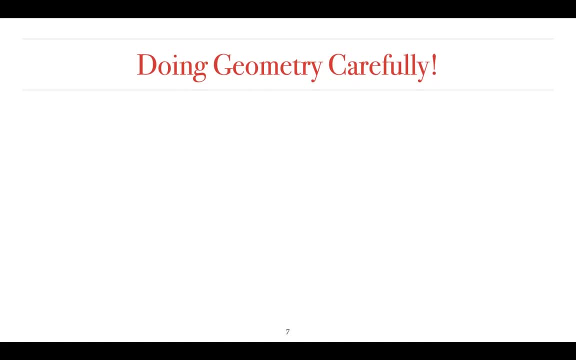 that, or perhaps only the logic. So of course intuition is very important, but sometimes intuition may deceive us. So if it is better that you should somehow- how to say that? convince yourself with the help of logic as well, 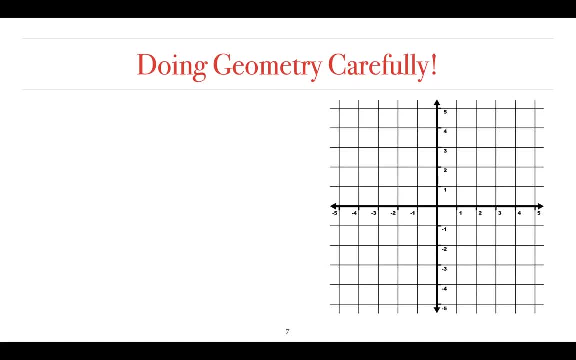 So now, in these cases, we will consider so, because we will always, because the 3D cases are very complicated in order to imagine. So we will start with just the 2D cases. So these are the cases in which, in which bug is studying the surface on which the bug is lying. So here I have. 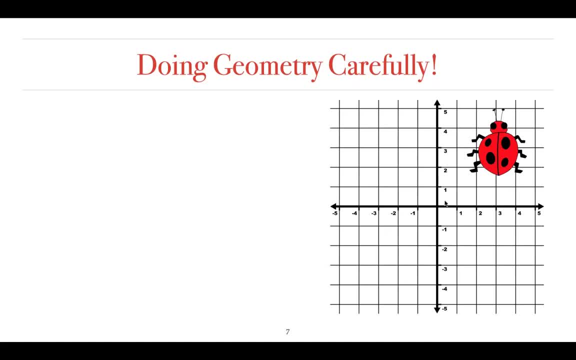 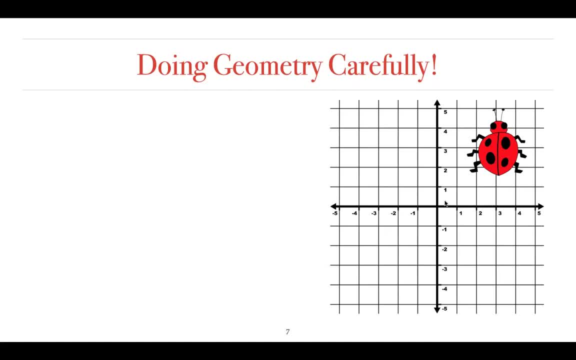 cannot look upward and it cannot really take help from navigation satellites etc. Okay So, okay. So now we have the basic geometrical notion. So one is drawing straight lines, Like how do we draw a straight line? So, and we will show next, or we will discuss next how to how we do this- 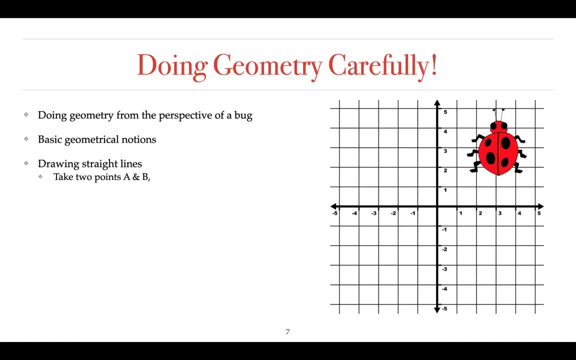 So the idea is: take two points, A and B, say any two points A and B, and find a curve of shortest distance between them. So this is how you draw a straight line And how would you draw a circle. So for that you fix some point which is called the center, and then you mark points at equal distance from that center C and you just join all those points. 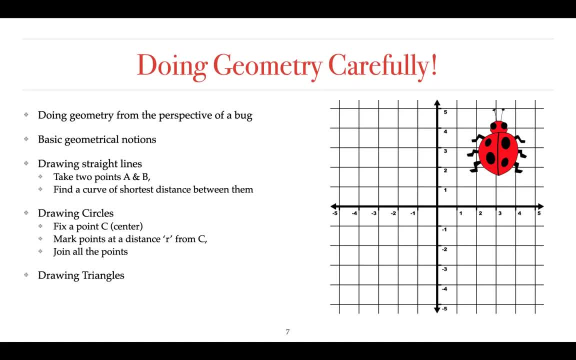 Then you will get a circle And also you can. so, once you know how to draw straight lines, you have to just fix three points And then, with the help of- because you know how to draw straight lines, you can draw triangles as well. 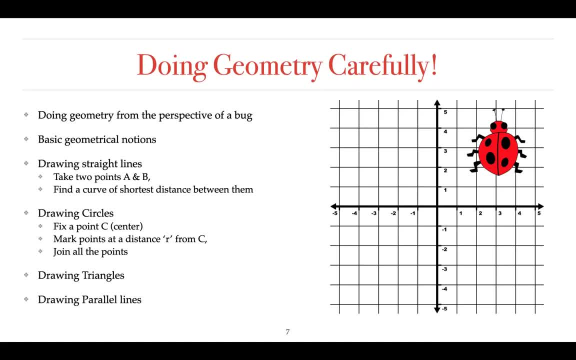 So now, and yes, And, And, then we will also see how to draw parallel lines, because, so this is one more difference. So, as we will see that, because this was a version of play fair axiom, So what I said was that if you have a straight line and a point that is not on the line, you can only have one parallel line. 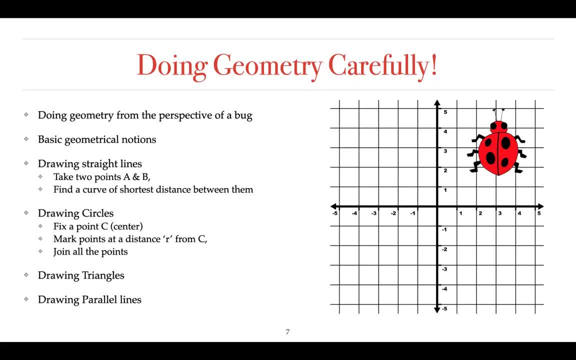 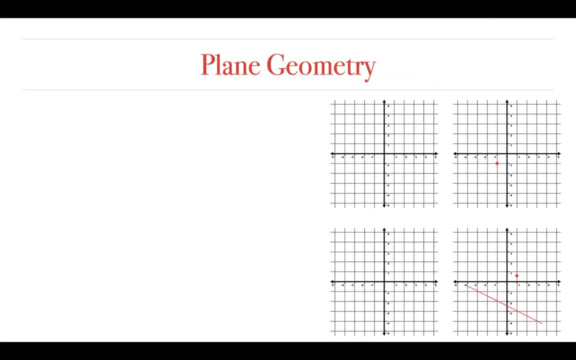 But, as we will see, this won't be true for the elliptic geometry and the hyperbolic geometry, as we will see. Okay, So now let us start with the plane geometry, the usual plane geometry that we are very, very much aware of, very much familiar with. 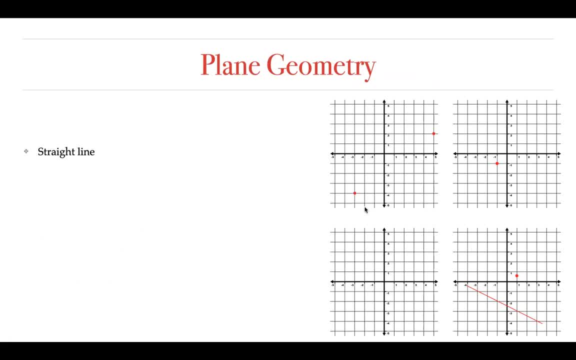 So now, how would you draw a straight line? So for that you will take two points. let's say here which is which has a coordinate of minus three, minus four, And this is five, two, And then you, you just draw a straight line because you, you just use a straight edge and just use a pencil and draw a straight line. 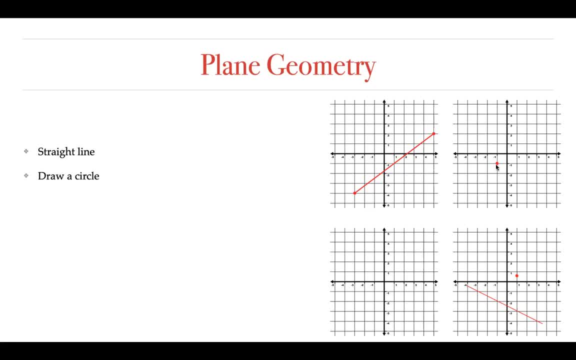 Okay, And now, how would you draw a circle? So let's say you have this point, fix C, which is the center, at minus one, minus one, Okay, And then you mark four points which are equal distance, equally distant from it. 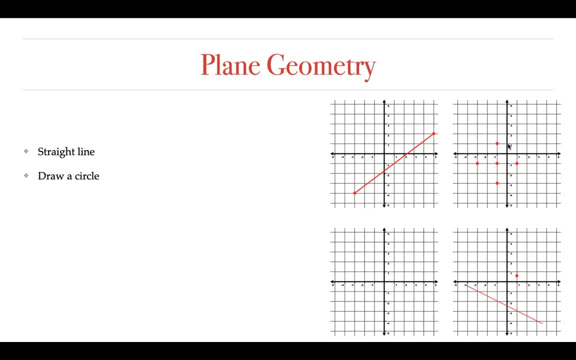 So one, two, three, four, These points are equally distant from this point, And then you just join all these points smoothly, You get a circle. So but? but there's a peculiar thing, or not, not rather peculiar, but but a pattern in all the circles. 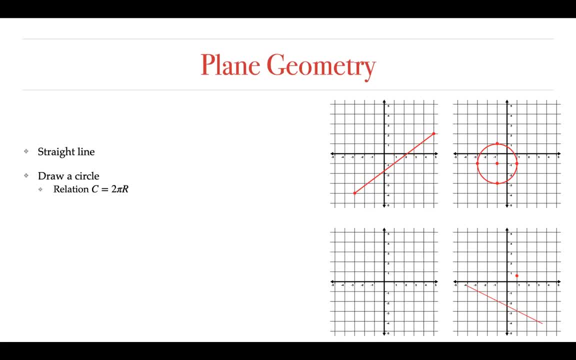 So, although you may draw very big circles, very small circles, whatever, whatever, but then all of the circles will satisfy one property: That the relation between this length, the total length of the perimeter, and the radius will always satisfy a given relation, which is this: 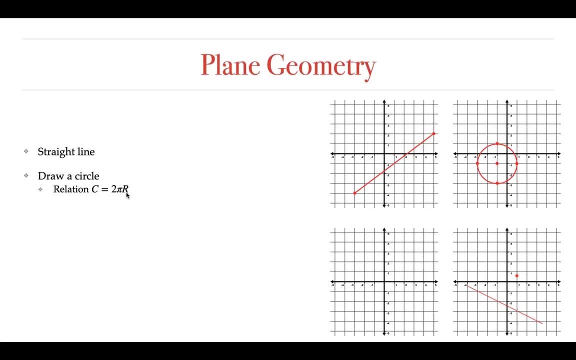 So it will. so there will always be a fixed ratio between circumference and the radius. So this is very important aspect of plane geometry. You will always find this. And next, how would you draw triangles? So for that, you will fix three points. 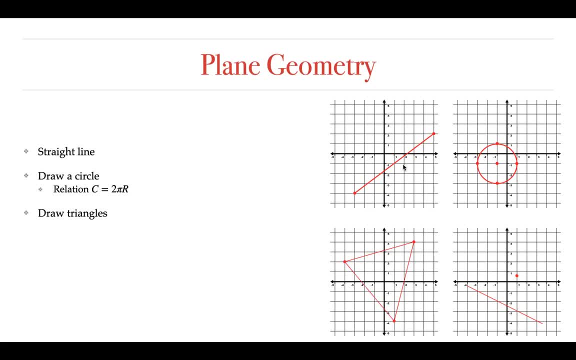 Let's say A, B, C and you just draw, because you now draw, now know how to draw a straight line. You can take three points and you just draw the straight line, And, and, and it turns out that the sum of the angle in all the triangles, in whatever triangle you make, it will all it can be isosceles. 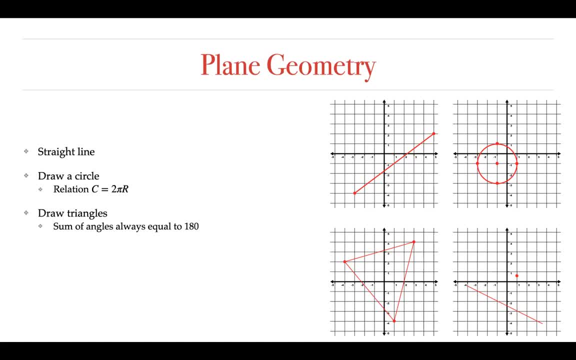 It can be scale in triangle, It can be collateral triangle, but the sum of the angles is always equal to 180 degrees. And how would you draw parallel lines? I mean, okay, Of course there's, there's a way of constructing parallel lines as well, but let us not go into that. 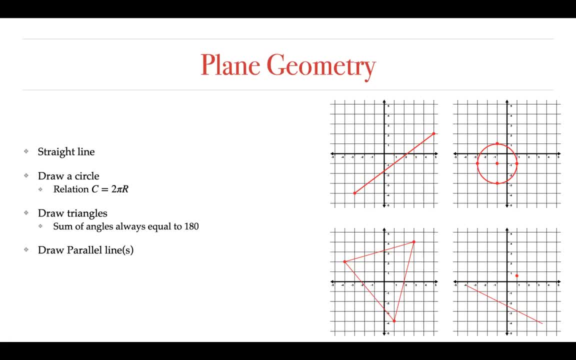 Because you, you can, if you want to, you can have a look at it in any geometry book, Or maybe I can say something about that. Okay, So, but but the point is that you, you will have only one parallel line, not more than that. 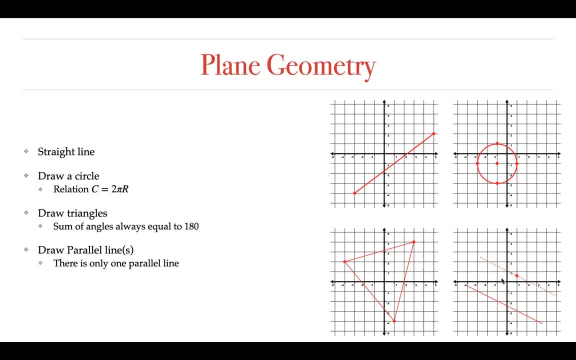 So if you try to tilt this line, it will eventually intersect. So so that's not the point I mean. so the point is not how to draw the line, but the thing is that there can only be one straight line. 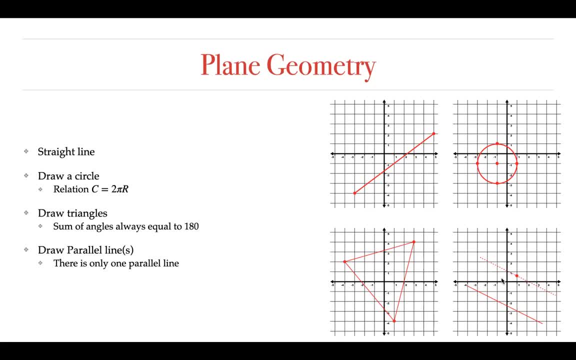 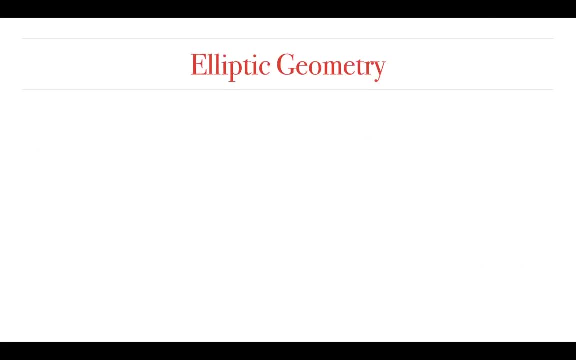 Okay, So, but okay, So, this one the case for plane geometry, but now let us, let us see what happens, or what differences are there in the case of elliptic geometry. okay, so, let's, let's draw a straight line. so one example of elliptic geometry would be the geometry that you would do in the surface. 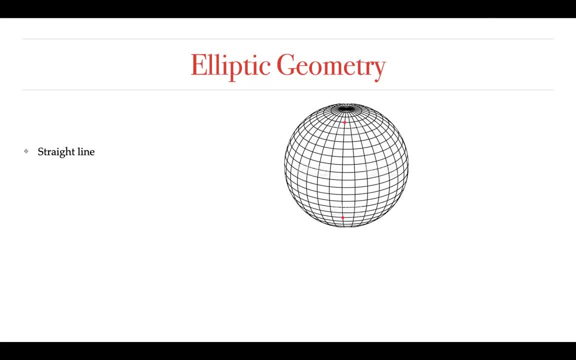 of a sphere, so no, so now. now let us draw a straight line. so so you fix two points here again. so let's say here and here and but now the but, now the straight line would be along the surface. it will not go through the surface because, as you remember, the bug can only because 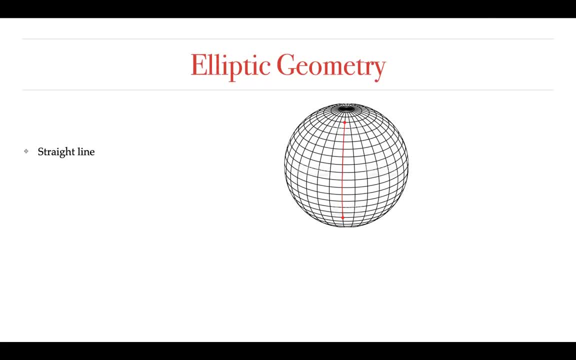 we are doing all the geometry with respect to, or the bug that is, that can move only on the surface. it cannot go upward, it cannot go inward. so this is the shortest line that is on the surface and this line is the is lies on the great circle. so if you assume, 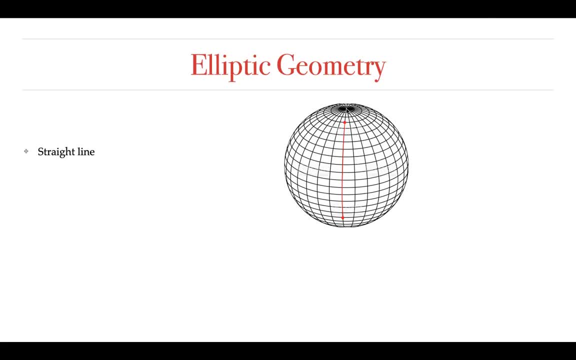 that this is. this is a longitude. so if you assume that this is a longitude, let's say: this is longitude, this is not pulling, this is south pole, so this line, uh, so this is a kind of circle that passes through the north pole, in the south pole, and and it and. 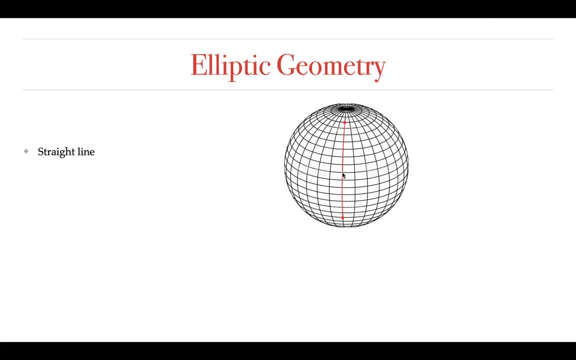 and this is the intersection, and the circle is the intersection of the sphere and the plane that passes through the center, not for in the south pole. so so this line lies on the intersection of that plane and the sphere. okay, so now you know how to draw a straight. 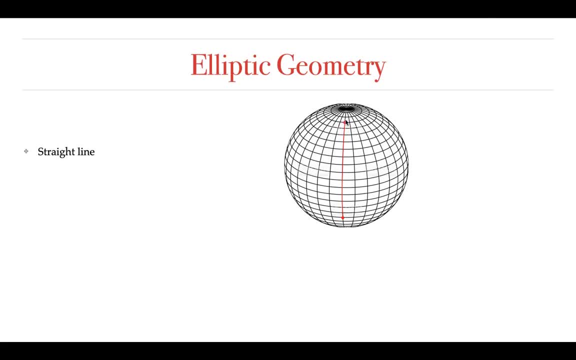 line. possibility was: could have been this. I mean in this way I'm not able to show it here, but, but you can imagine what I'm saying- but that would not have been, but that that would not have the shortest length. so because in that case the length would have been more as compared to this case. 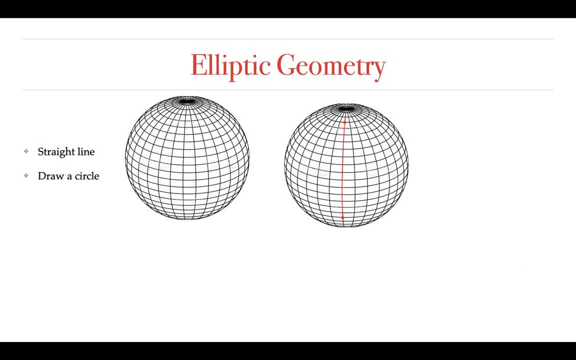 okay, so now, how would you draw a circle? so, for circle, let's say you fix a point, because now we are using the definition. so you fix a point, let's say this is your point, and then you measure distances which are equally distant from this point, here, here, here, here, here, here. so all these, 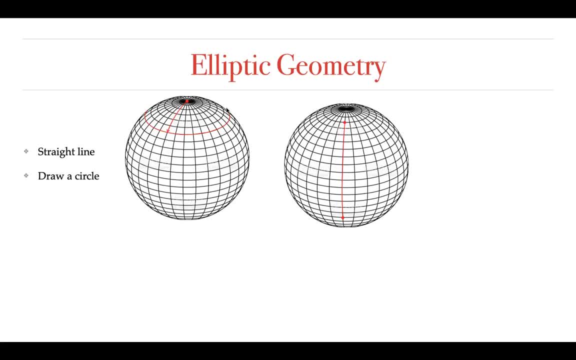 points are equally distant from this point and you join all these curves, all these other points smoothly, and then you get a circle. so now you see some peculiar property of this circle. so this circle has different property from what we had in the plane geometry case. in this case, 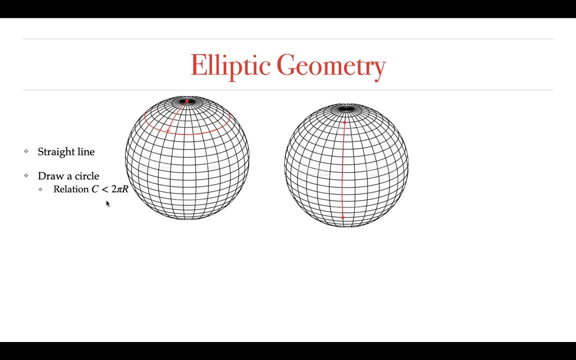 you will find this relation to be true, that the circumference is always less than 2 pi R. and why is this true? as you can imagine? because, and as you can imagine this, I mean, okay, so, I should have taken that diagram as well, okay so? so let's say this is the circle, but how to say that? 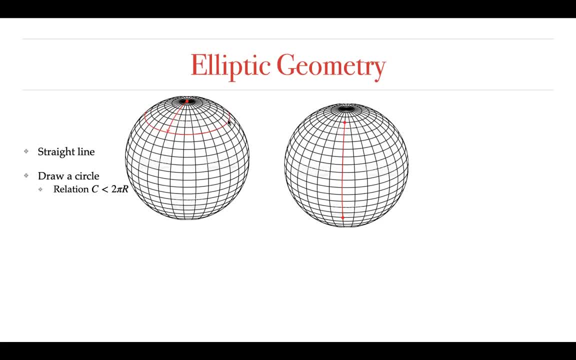 okay, so. so I should have put a picture, but but anyway, okay, so. so I'll explain it in some other, some other days, because it will be. it would not be easy to explain because I have to make some, or maybe I'll explain in that with the help of some diagram. okay, so, now, how? now, how would you draw triangles? so 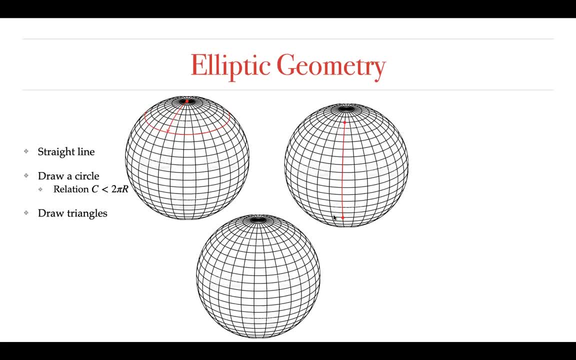 so here we learn how to draw straight lines. so one thing to be remember is that you have to put your straight lines only on the great circles, so they cannot be elsewhere. so once you have, let's say, got three, got three points. one is on the north pole and this is these two are on the 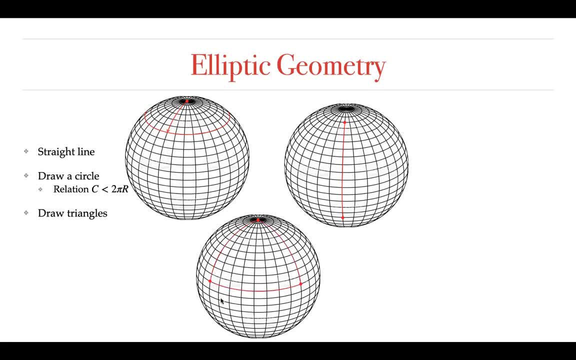 equator. so now you just join them together in this way, because- and this line will lie along the great circle, that is, a circle which is which is on the intersection of this sphere and a plane that passes through the center and these two points. is this clear? 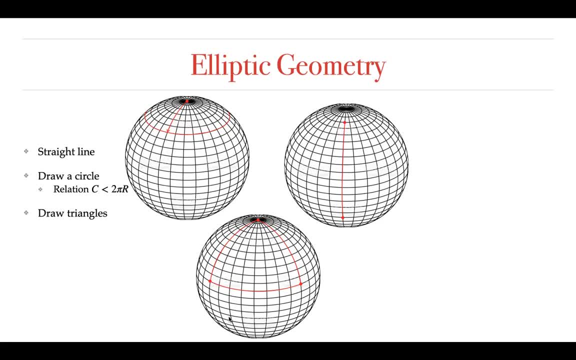 am I audible? yes, sir, yes, sir, you are clear, sir, and and is this clear what I'm saying here? yeah, I'm trying to, okay, no, so the thing is that, um, okay, for for this case. so you, so you should always think about great circles. so great circles are the circles which are obtained. 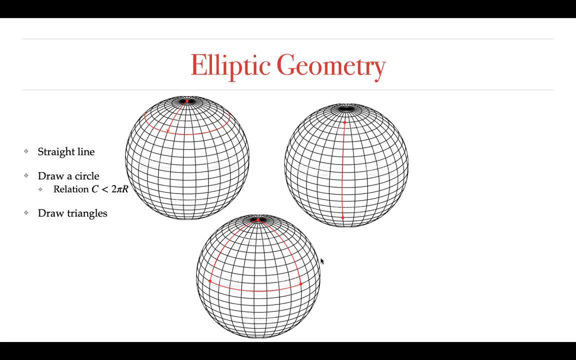 when you intersect the sphere, the whole sphere and a plane that passes through, let's say, these two points and the circle, which is the center, and the whole sphere, which is the center and the whole center. so three points will uniquely determine a plane. so you will get this. okay, I should have. 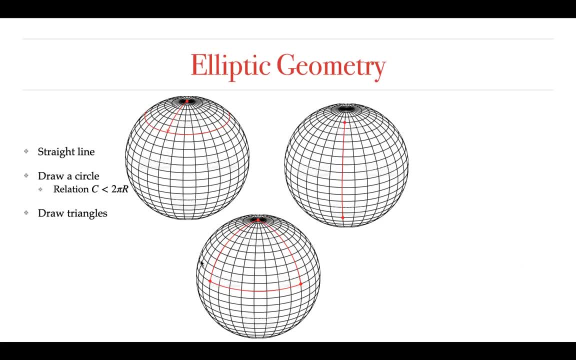 also put a picture, but but okay, anyway. so this line will lie on that circle and this circle is known as the great circle, because this will have the greatest radius, greatest possible radius, because if you think so, so you. so you could have said that, why not this? let's say why not this? but 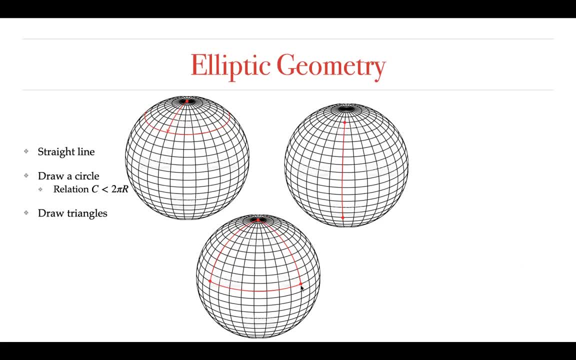 this won't be having the shortest distance, so this won't be so. this won't qualify as a straight line, as per our definition, but in this case you will find so. in the case of plane geometry, you found that the sum of the angles is always equal to 180 degrees, but 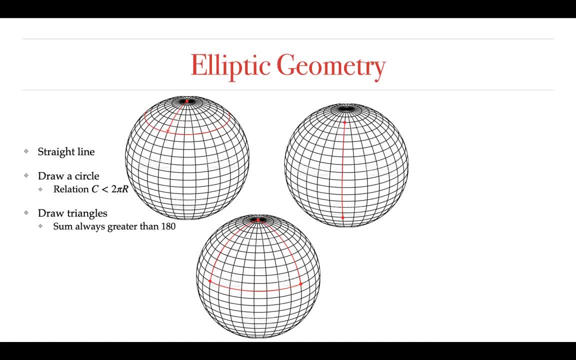 in this case, you will find that the sum is always greater than 180 degrees, as you can see here, because you see, these are almost 90 degree angles. so this is 90, this is almost 90, this is almost 90, so or maybe perhaps let's say 80. so if you add 80 plus 80 plus 80, you will get. 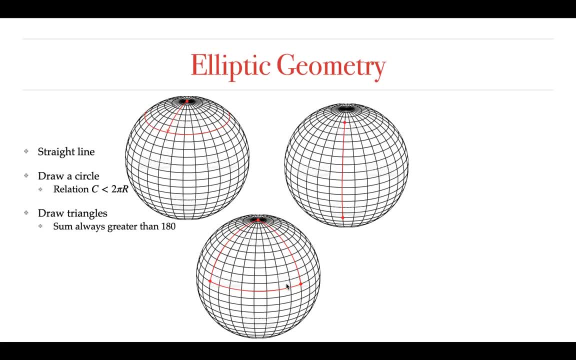 240, which is definitely larger than 180.. so in this case, it's in this case, all the triangles, all the triangles- will have to have the sum greater than 180 degrees and the larger the triangle, the larger will be the departure from 180 degrees and, as you can show, if you do some 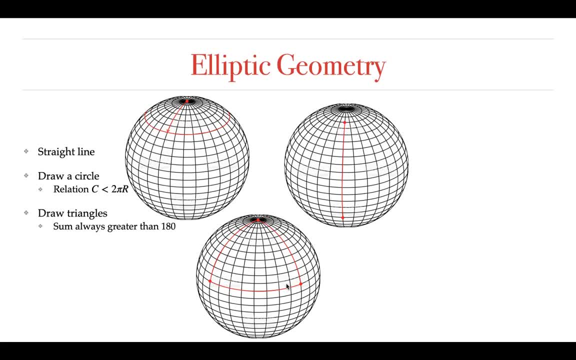 math. you can. you should be easy. it should be easy to show, or there are reveals available already. you don't have to derive them, just have a look at them. and now, how about drawing a pattern line? so let's say, this is the line that runs from north pole to south pole, and this is the point. 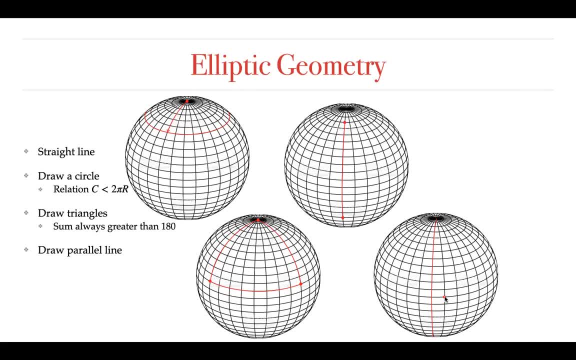 through which we want to draw a parallel line. but is any parallel line possible? can anyone say the answer to me? no, no, i don't think so. i don't know, because it will always interact, sorry, it will always intersect at north pole and south pole, but but one thing yes: 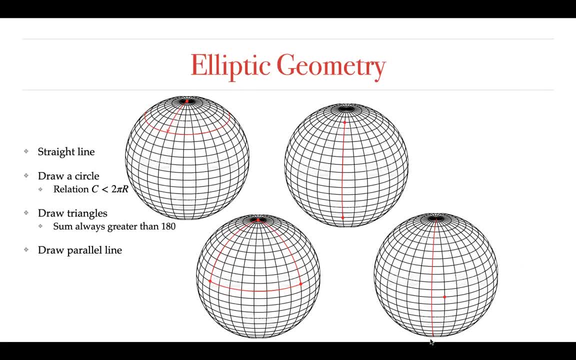 a pattern. this has the radius of, let's suppose, edge of the universe. so by the time they will intersect, they will intersect at the edge right. sorry, sorry, what was that? let's suppose the radius of this great circle is: is the edge of the universe, or you mean the, uh, the radius equal to the visible? 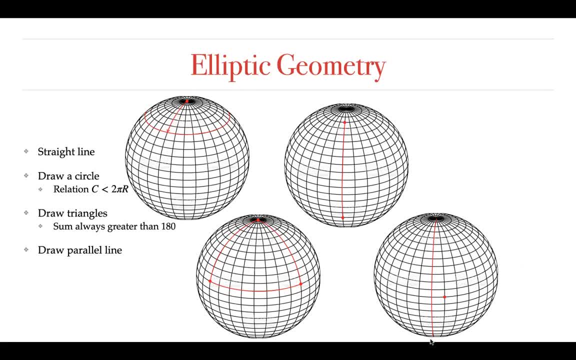 uh mode, yes, yes, yes, yes, at least visible universe, okay, visible universe, okay. by the time to, let's suppose we draw two line. of course, in principle they will converge at the point. what is that called? north pole or south pole? okay, but now imagine you're actually. 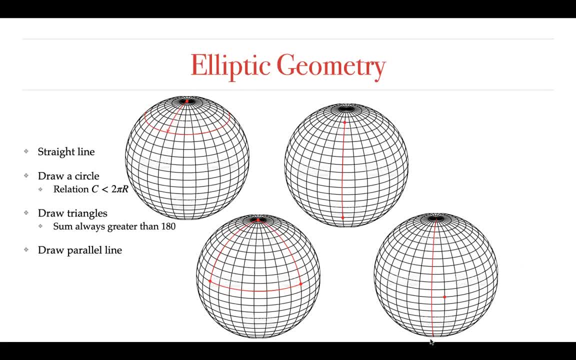 treating it like much bigger, much bigger great circle or sphere. so the parallel line will intersect at the edge of the universe and they will be like, but i think the angle between them will change right. so concept of parallelism never exists in this geometry. yeah, so i did not get your question. what you're asking, i did not get your question. 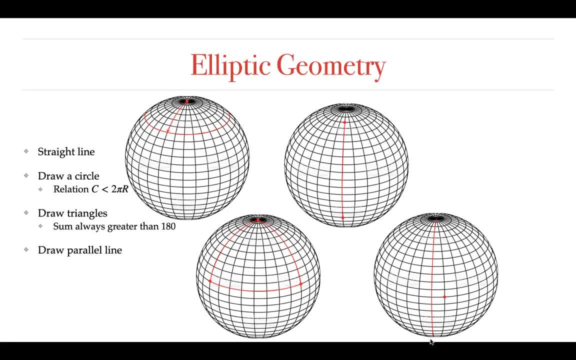 what i'm telling, that the the concept of parallelism or the existence of through parallel line, i think don't exist in principle in this kind of geometry. yeah, yeah. so this is what i'm saying because it will always, because this will be the straight line that passes through this point, and 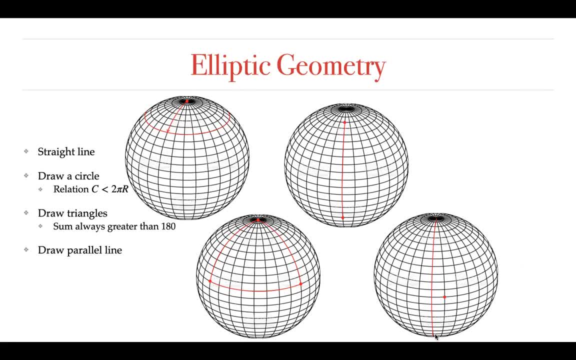 it will intersect at north and south pole, if you can see. also, if it doesn't intersect, also, if you see the point to point the distance between two line, actually it does marry parallel lines means the distance between two lines has to be even fixed. no, no, that is not. 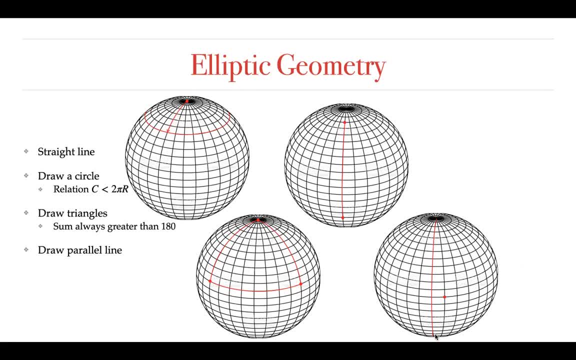 true that is. that is not true. i mean that, that that is perhaps so, so that is an extra assumption or that is something extra that comes in the case of plane geometry, but it is not true in general. no, i mean what i'm trying to say, if you see it, or can you see my course? 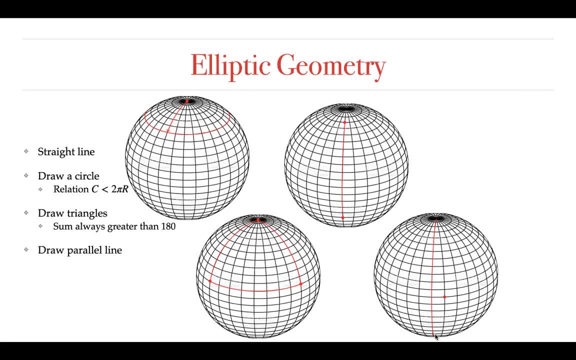 i can, in the last, last, last great circle. okay, okay, okay. so you have drawn a line and you are asking for the parallel lines. okay, so now, if you see, let's suppose in plane geometry, of euclidean geometry we used to call, two lines are parallel, provided the distance between them remain constant. 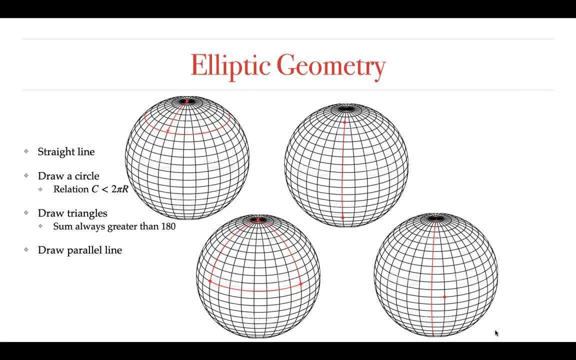 No, you see, you have to understand one thing here. I mean, perhaps in the case of Euclidean geometry, the parallelism will imply this, but this is not the universal definition of parallelism. Exactly, exactly, exactly. But here one criteria. you are saying. that is correct, of course. 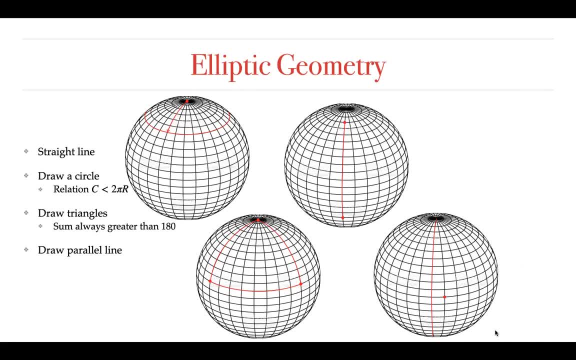 that if you see two lines they will meet either at the north pole or south pole. Correct, But from the great sphere- sorry, that is called great circle if you just go just one centimetre up or one centimetre down, or one kilometre up or one kilometre down, the distance 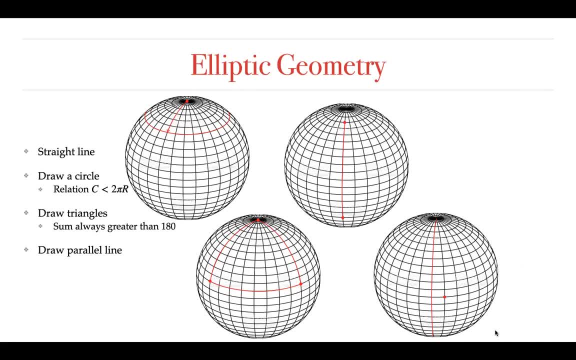 between them also vary. That says actually they are converging, right, Okay. So from that cannot we conclude: Do we need to see the end points? Yes, that may be, because, as you will see, in the case of hyperbolic geometry the distance 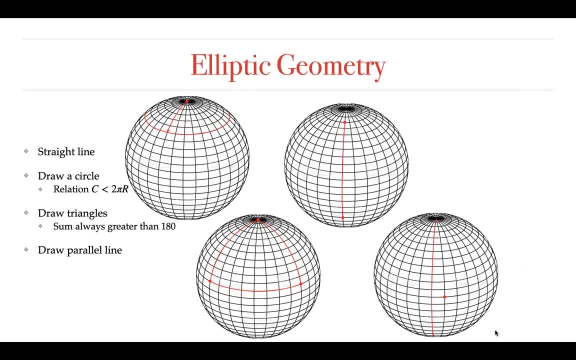 can also change there. But, yes, in that case the distance always increases as you move away from the point. So, yes, What I mean to say it will not remain constant immediately If you, however small may be the variation on the line, if you just go up or down by a kilometre or metre or centimetre. 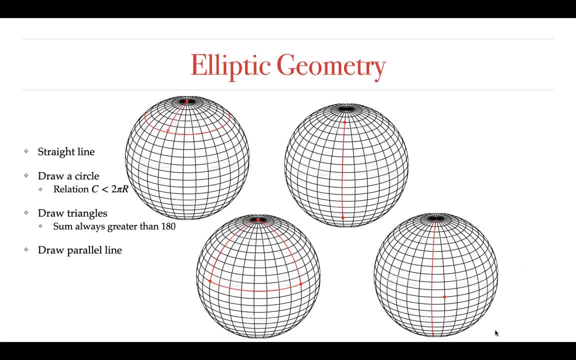 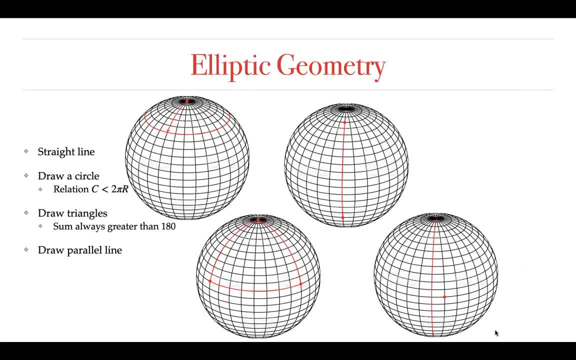 we have not done the Euclidean geometry. Okay, Yeah, fine, I mean so. so. so then you have to add one more. I mean add one more detail to it, that the, that it is not just that the distance between the, let us. 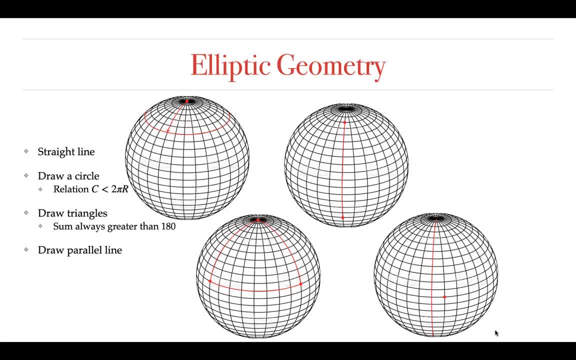 say the line point, Okay, The distance changes as you move away from the point. You also have to say that the distance should, in should, increase if the line were to be parallel. If the lines were parallel, the distance should, as you will see next, because in this case the distance is decreasing. 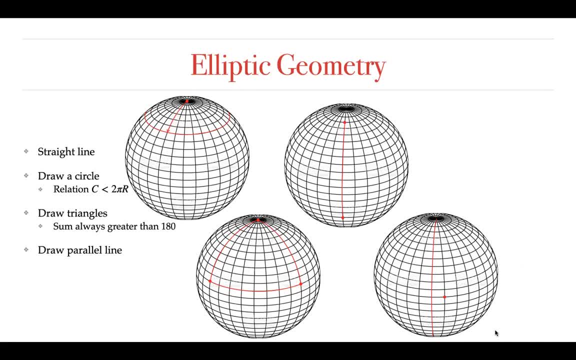 but in the case Yes, Oh, sorry, I am sorry. I am sorry, I meant in this case the distance is decreasing, but in Yes, So so, yes, So so, eventually they will, they will meet at some point, but that will. 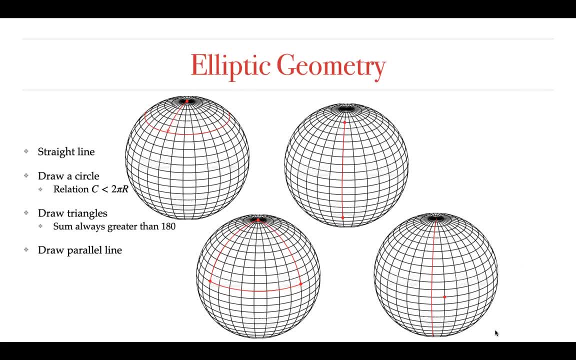 not happen in the case of hyperbolic geometry, because in that case also They will receive that one from each other. Yeah, yeah, yeah, Okay. So positive geometry case, Yeah, I mean so. so so this is positive curvature case and that is negative one, Okay. 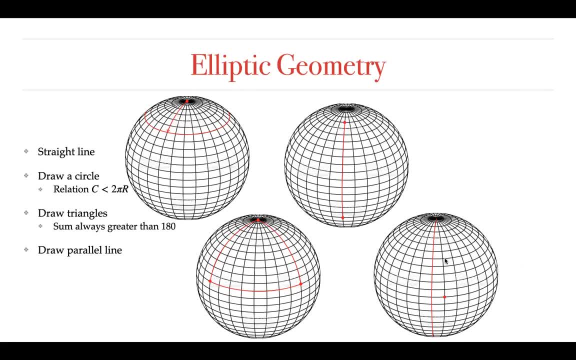 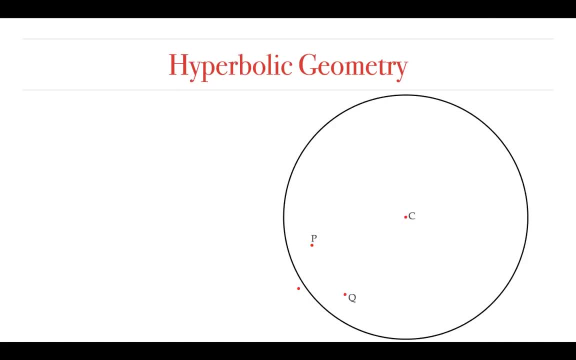 Yes, yes, Okay, Fine. So so, in this case, as I, as, as we, as we saw that there are no parallel lines, but now what happens in the case of hyperbolic geometry? So so, hyperbolic geometry. 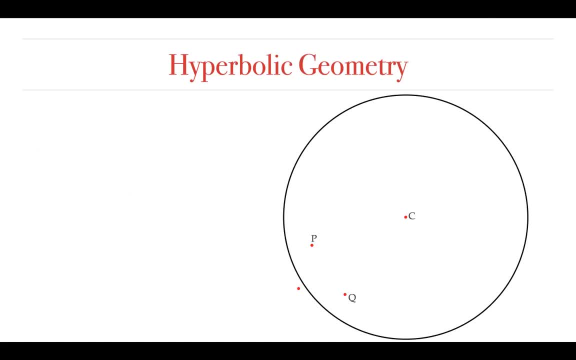 is a bit difficult to imagine, But then many mathematicians have come up with a model, So this. so this is known as a Fonker. it is So we'll. so we'll consider this example. So so this is something called. 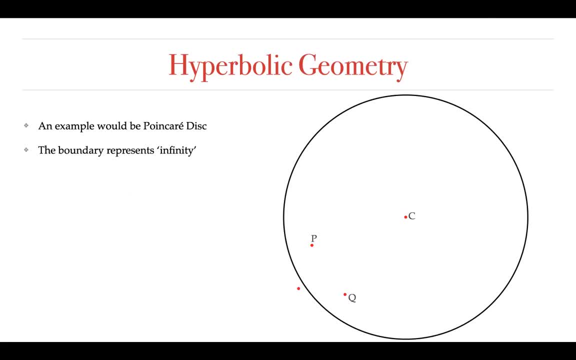 as a Fonker, it is So, so in, in that case, what happens that? this boundary, so this boundary, represents infinity, So you can see infinity here, Okay, And this is the, this is the center of the circle, and this and the boundary represents infinity, And the objective is to find out. 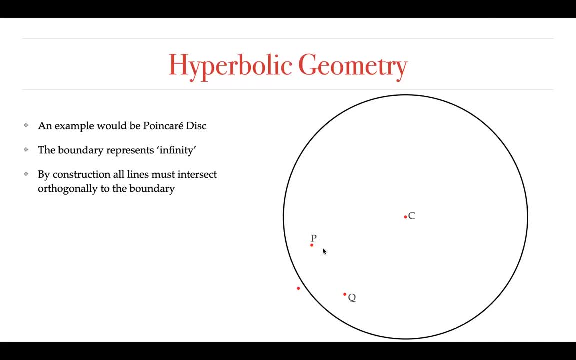 a line that is per that goes through PNQ. Okay, So now we will show the construction of me of of making or drawing a line that passes through PNQ, because, as we said before that this is the most basic requirement of a geometry: that if you are given two points. 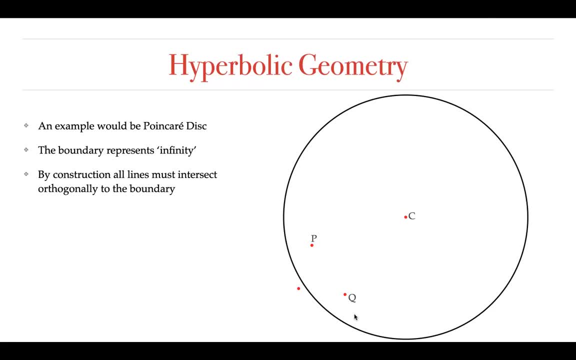 you must have a way of drawing line through them. Okay, Okay, So how would you do that? On end: Yes, There is one more requirement. Okay, So, if you can draw this, this line, I mean, perhaps this comes from the mathematics itself. I mean, I am not so sure about that. 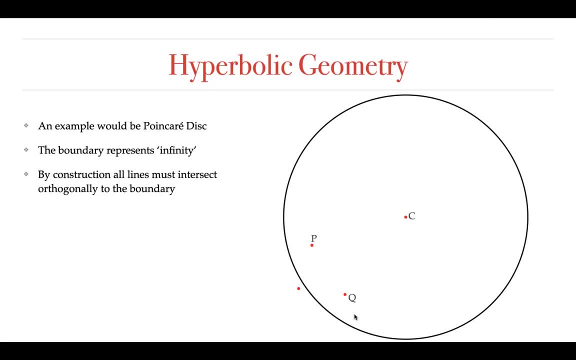 So I cannot justify, at least it right now. So the so one more requirement is that all the lines, so let us say any line that you will draw, let us say passes through point P, must intersect orthogonally. So and as I will say: okay, So let us say a line, there is a. 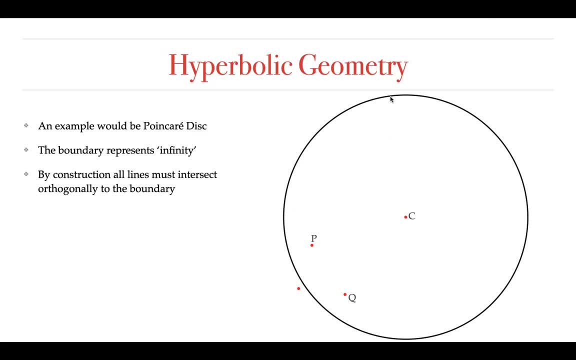 point P here and you have a line that passes through this. So this angle should be 90 degrees. Okay, This is the requirement. I mean, I am not sure how this requirement comes about, but okay, at least not now I am sure. but I should read about it and I will let you know later. Okay, So, 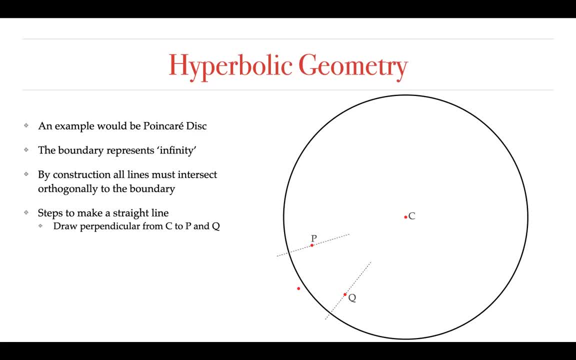 now let us see the steps of making a straight line. So first step is you draw, so this is center, and these are A2 points. So this angle will be 90 degree by default, because these are normals, because we know, in the case of circle, all normals are all normals passes through. 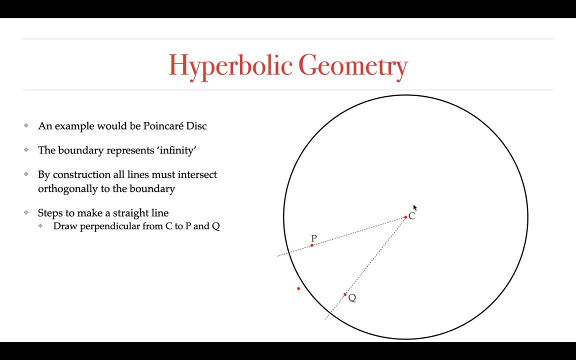 pass through the center of the circle In the case of circle, because circle is a very special kind of curve. Okay, So let us say, and I have, although I have not written down: let us say these points are m and n. Let us say this is m, this is n. So from m and n, now draw. 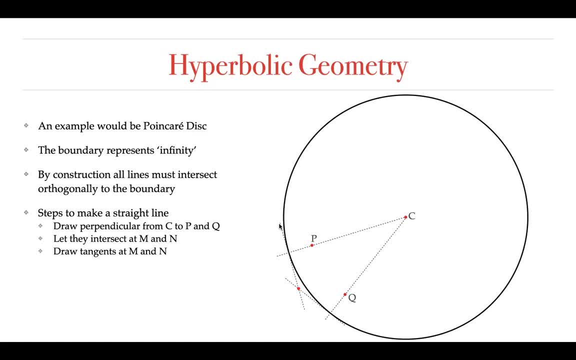 tangents. So these are the tangents. So this is tangent 1,, this is tangent 2, and let us say these T is made at some point S, This is the point S, And now from S you draw a circle which. 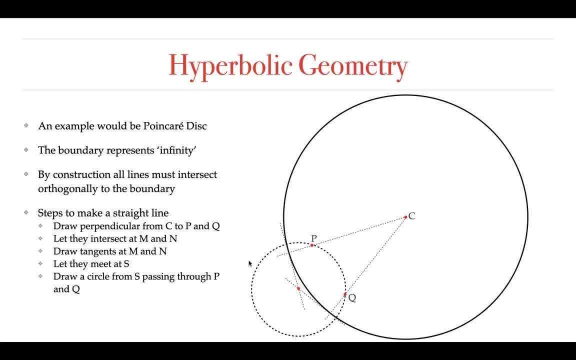 passes through both P and Q. So in this way, So this is a circle that has P and Q on its circumference and S as its center, And now your line is this: So by construction, we have ensured that this angle is 90 degree, And this is your straight line in the case. 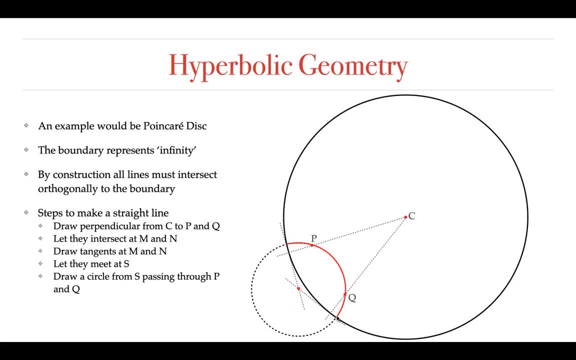 of hyperbolic geometry. Okay, So once you know how to make a straight line, and similarly, you can also use the relation or the definition of drawing circles as well. So now, once you know how to make straight lines, you can draw triangles, etc. And if you do that, you will. 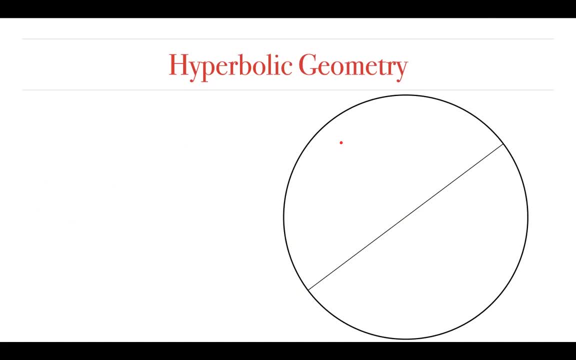 find that there's some. Some of the three angles of a triangle is always less than 180 degree. Okay, And for the case of circumference? so this is what you will find: that the circumference is always greater than 2 pi r, as you can check, And the sum of the angles of a triangle is always: 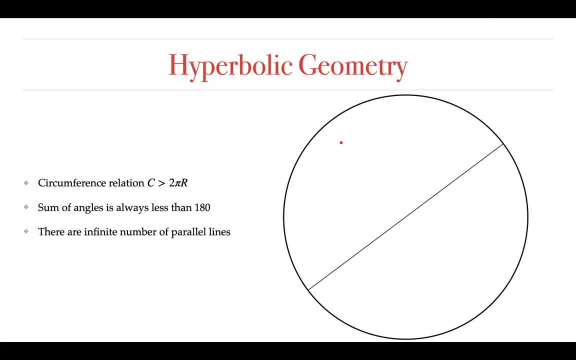 less than 180 degree And there are infinite number of parallel lines. So, for example, so one line can be this: I mean, this is not exactly perpendicular, but this is perpendicular. This is kind of geometrical problem, but yes, But you can do this. So this is one. 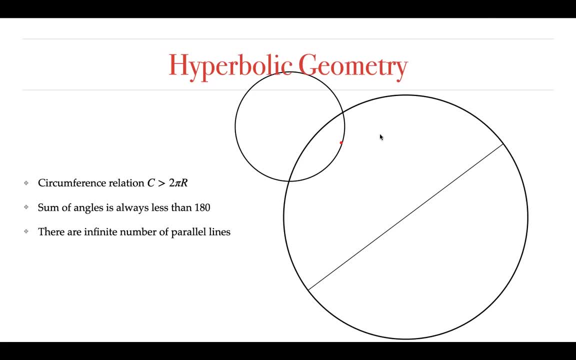 line. So let's say: this is the line And this is the point that is not on the line, and we want to draw parallel line to this. So, because this is infinity, they cannot go anywhere. and this is a line, this is a valid line. So one line is this: this is: 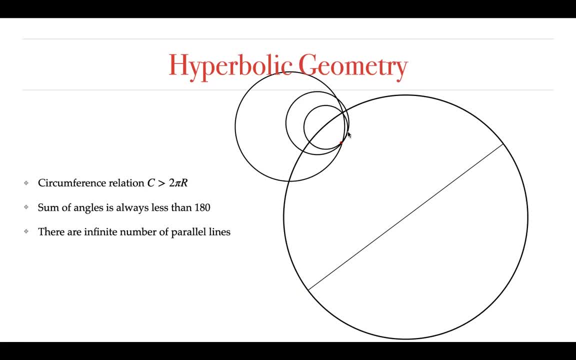 another line, this one, And this one is another line which passes through this. So these are all parallel line to this, So you can have infinite number of parallel lines. So now let us summarize and conclude what we So. before you summarize, I just want to ask a small thing. Can you go back? 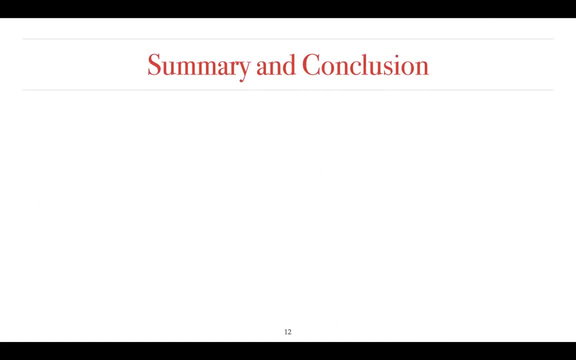 You have drew some parallel lines, the small circles, So clearly in the correlation point it is portraits, But what you are focusing on is parallel lines, or the squares or the tiles. Yes, I mind my不錯 a little bit generalいて, as you mentioned thatiels, it is not. 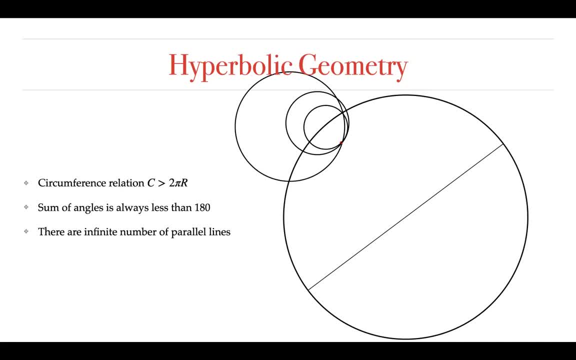 context of our physics, or we will be discussing this in terms of the curvature. okay, so we're still, though we are starting it in the abstract viewpoint, but if you just consider two things, the suppose you are living in a curved universe or a curved space time, and the scattering is happening. 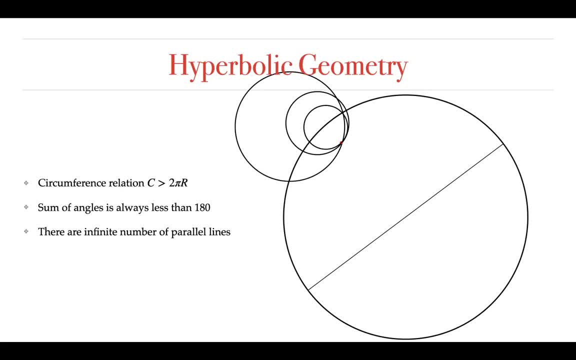 and if suppose the scattered, particular, simple, following the trajectory based on the curvature they are actually relying, residing here, cannot, they, cannot they actually give us the hints that what is the nature of the curvature of space, time the scattering has happened, let's suppose, as you said, in the circumference of the circle or the some of the angle of triangles. 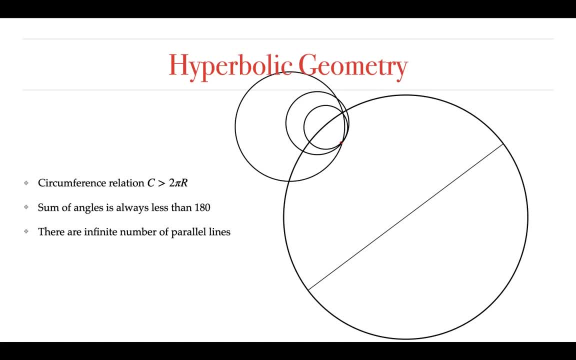 that essentially decides whether it is positive getting across geometry. okay, it's supposed to do this with each other and they simply followed the trajectory based upon the space time. okay, they cannot randomly move that. okay, so, depending upon this angle of incident and under scattering, uh, so cannot we actually draw any sort 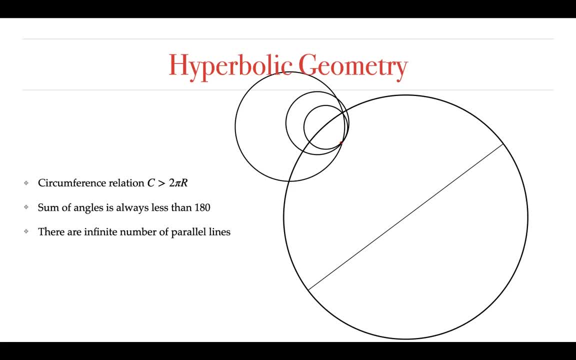 of fields or indication that you have sort of geometry actually on upon which the scattering event was so, uh, so, so, if i'm correct, i mean i, if i, if i get a question correctly, then uh, so, perhaps, so, so, please confirm, i mean so, so there's one more way of simplifying your question, so, so, so one way i mean. 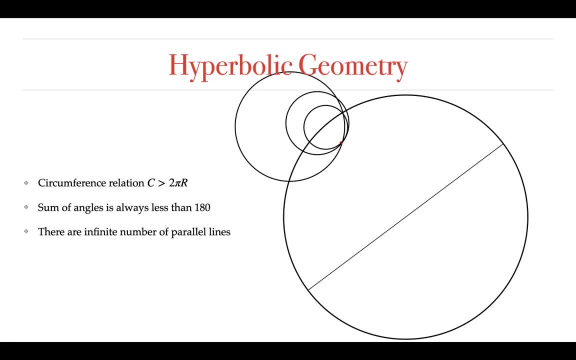 why look at, uh, the particles? perhaps the perhaps one more way of, or perhaps a better way, is to just draw very, very large triangles and to see whether the some of the triangles of a triangle is or not. that is perfect. that is perfect, but i am just saying for the sake of curiosity. that's a very 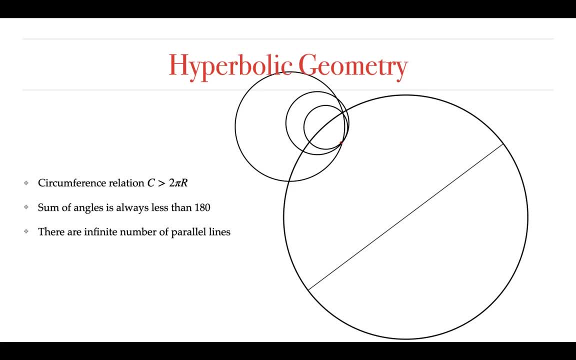 uncomfortable scattering event is going on. so let's suppose you are studying it in more details. let's suppose in shorn or formula forever. so we are calculating this weinberg angle fix mechanism and all that. so cannot, uh, information about the space time be known from that event? it's, it's very. 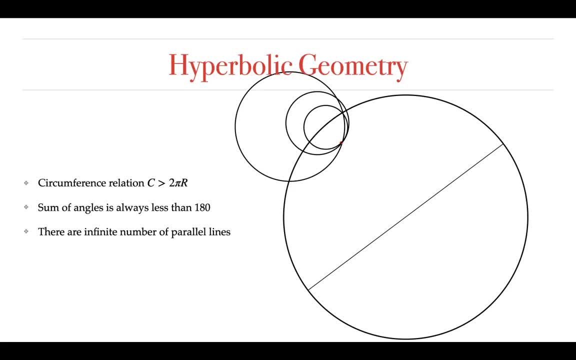 unlikely, because, you see, i mean so, the, so the information of space time will okay. so so now, as we know that, according to general relativity, the uh space time gets modified because of the presence of matter and mass in it, so so it may get modified um it, it will be modified, but the modification 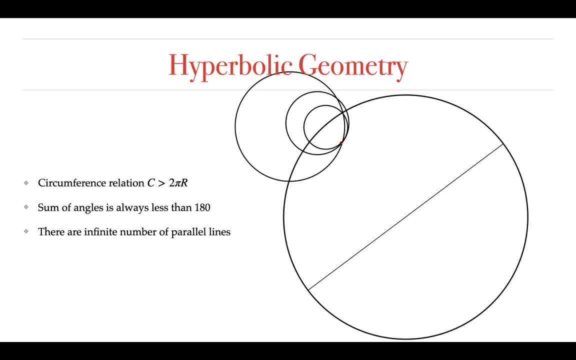 is so small that it is barely detectable, because the most of the effect will be because of Earth's gravitational force or because that's the whole thing. honestly, you just have to be careful of the. obviously you have to be very careful because actually that's not the same thing as if the 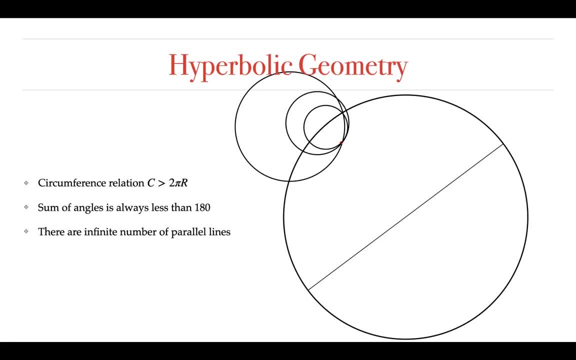 gravitational forcehalt will be wondering about it and you could just go down and look at it. this that's of earth's gravity. that would be very small, at any rate. so how would you even see that? how would you even detect that? yeah, whatever you say, it is a challenge from the technical side. i i means our- 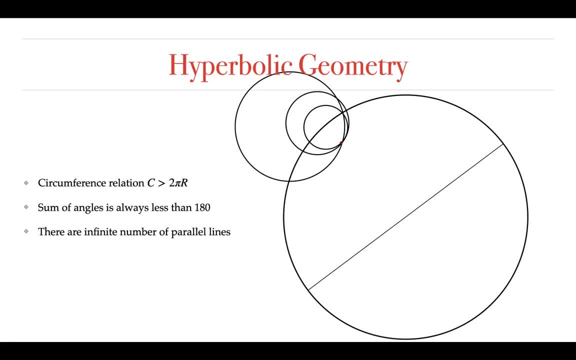 precision problem, but in principle we can get any sort of information regarding the background space time, right on which event is occurring. but it is possible. but yeah, i, i guess in principle it should be possible. i mean so. so one one easy way would be to just see how much a photon deflects as as 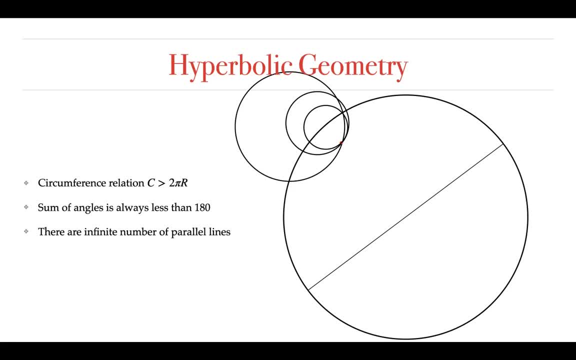 so let's say you are pointing a laser in in the horizontal direction and, and, and, and the, and the lasers propagating, or the, or the photons are propagating, and and. by the deflection that happens to the laser at some distance you can also infer something about earth's gravity. 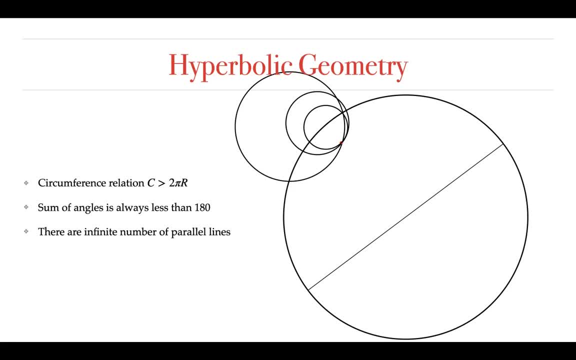 so finally, okay, okay, maybe, maybe, since we have a lot of theoretical and experimental knowledge right now in favor of gtr, so it may feel like. it seems like, uh, it's an easy buying problem, but during the early stage of gtm or by the time this concept would have been developed. 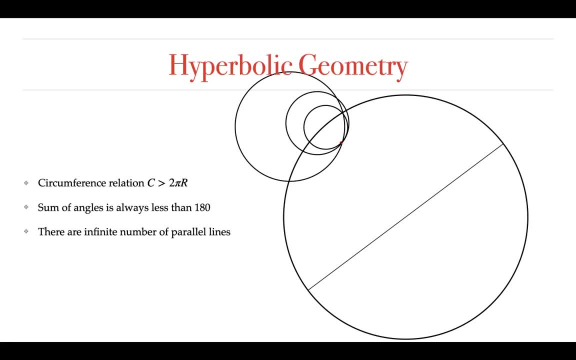 since before 2000 years ago or so. so it would have been an incredible way of studying the space time along this line. yeah, so i mean, one one very easy way of doing it is to: so, so you do the geometry on the surface of the earth. okay, so, so then you, uh, so, so, okay, actually i, i taught this at qwc. 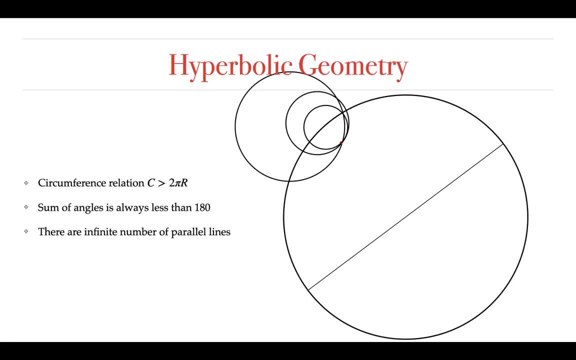 so i'm not able to recall what i said there. okay, so, so, so one way of actually detecting whether the surface of- uh, surface of earth is curved or not, you just draw big, big circles on the surface of the earth and you measure their radius, okay, and? and then you can also. 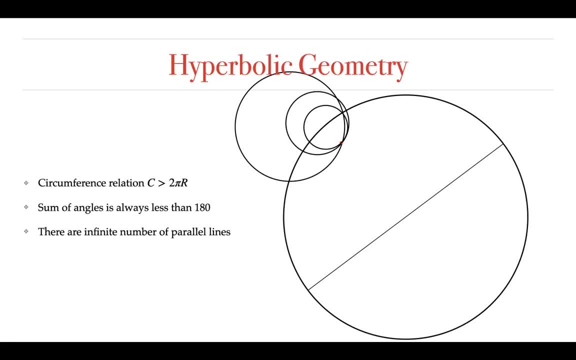 i mean, i'm not able to recall it right now. let me think a bit. so, oh, yes, yes, yes, fine, fine, also, yeah, so, so this is how it goes, so okay, so so you can measure two things. you, you fix the point, let's say, you fix the point on the surface of the earth. 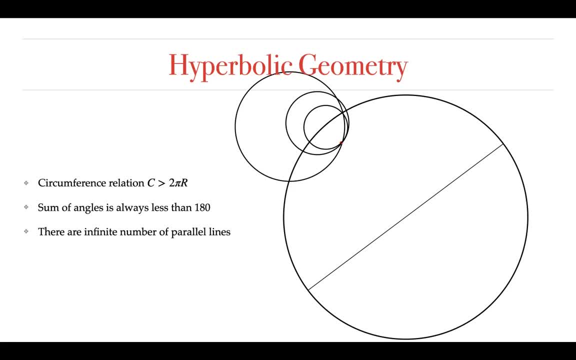 and, and then you draw a circle, a very, very large circle. let's say 20 kilometers of radius. so the circle is 20 kilometers of radius, and then you draw a very, very large circumference. so first of all you have to somehow arrange 20 kilometer long rope. 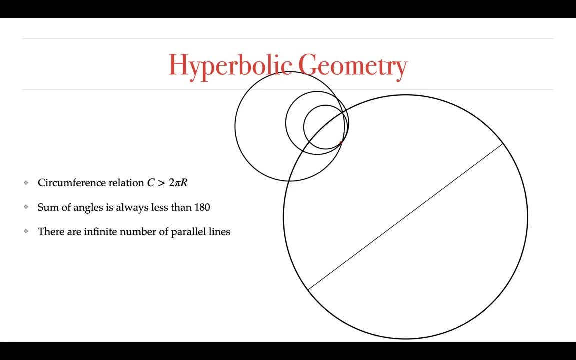 then only you can do this. so, so the radius is 20 kilometer, and then, and then you can also measure the periphery, the circumference, you will, you will find a deviation between the two. i mean, so the circumference should have been 2 pi r, but you will not. but, but, if you do the math correctly, you, if you. 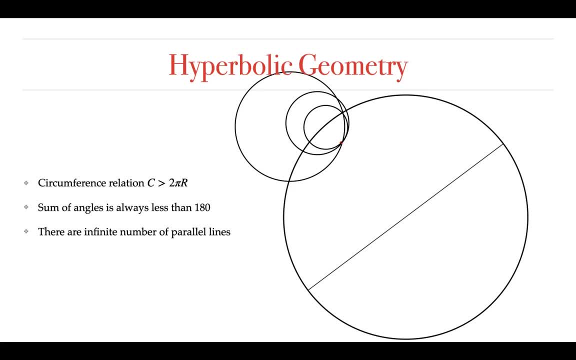 do the math there, you will find that the circumference that you find for the circle is not equal to 2 pi r. so then it will give you indication that this, that the surface you are living in, is curved. but one question then i would like to ask. maybe i just like to refresh my school. 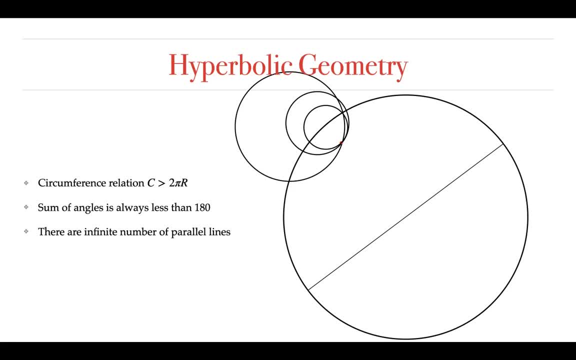 but by the time this element was discovered, people used to give the ideal example. how do you know that the surface of earth is curved, not still not flat? they used to give you many examples. like you can see the muscle of the, the back of the stick, from a very distant. 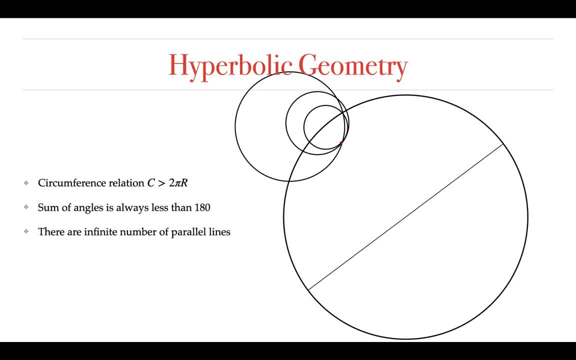 sea. so that is an indication. uh, clearly this is a school, school team knowledge. so this kind of concept, why haven't they used them? sorry, sorry, this kind of what was not done. no, as you said, the experiment is very simple because there are some objectives which actually stretch. 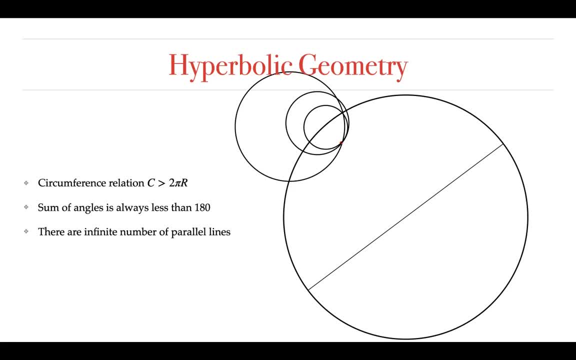 hundreds of kilometers. right, okay, so people can very well would have gone there and drawn a circle of 20 kilometers radius. it's not a big deal. but will you give the indication that they see less than, of course, less than 2 pi r, so they would have confirmed their excel before 2000 years ago. 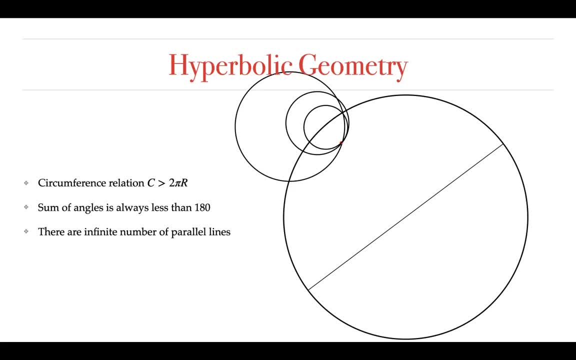 yeah, um, perhaps it's not. it's not worth the pain because first of all, you have to arrange. i mean, we are happy, we are not much concerned about the geometry of the earth. okay, okay, i i just why did i ask this question? because this is how we have actually 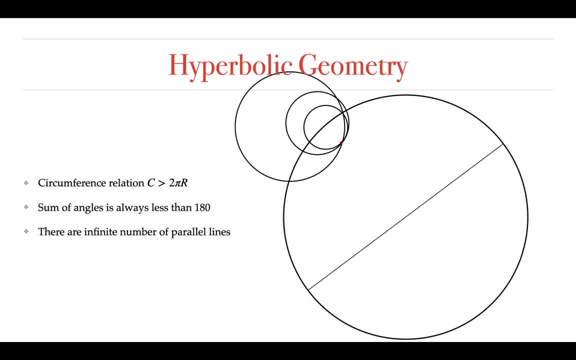 taught in the school and intermediate colleges. people used to ask the science, which are used to ask you the question: how do you know that surface? the earth is spherical, so we used to see. now from a distance? uh, from a distance, we can see the top portion of a sea in the deep sea. 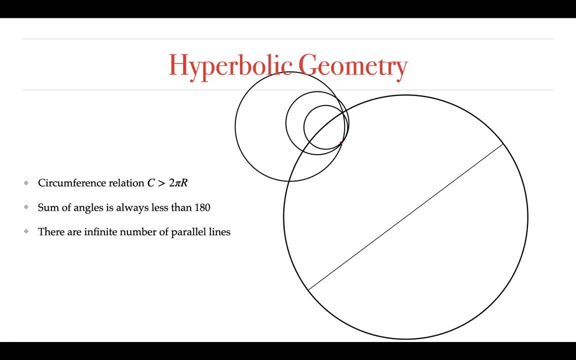 while it is approaching to the source. so why do i need to wait for a ship to appear in the deep sea? i could have gone very well through the desert, if at all i am staying in, uh, let's say, for that pyramid, that area i could have, i could have drawn a circle of the kilometer and would have measured, and the triangle. 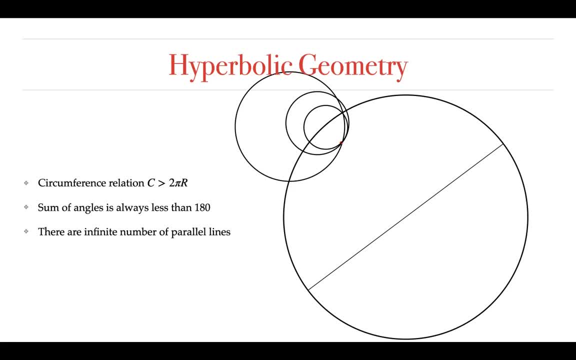 also any sort of thing have done. and this thing is so simple, because by then i don't know what was the standard of voyage, because she could not have been in the concept of, in the dream, actually, in this regard perhaps, uh, a greek mathematician, eratosthenes. so there was a greek mathematician called. 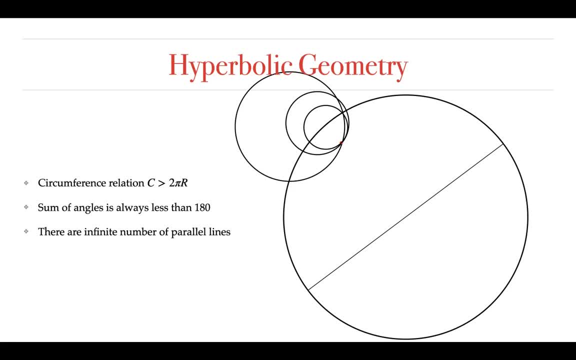 yeah, so so he actually knew and and based on this only, he kind of calculated the earth radius. so i mean he, he actually used, uh, so it's okay. i mean i'm not able to recall the exact experiment, but then he could calculate the earth's radius by seeing the shadow. that, uh, okay, so this is. 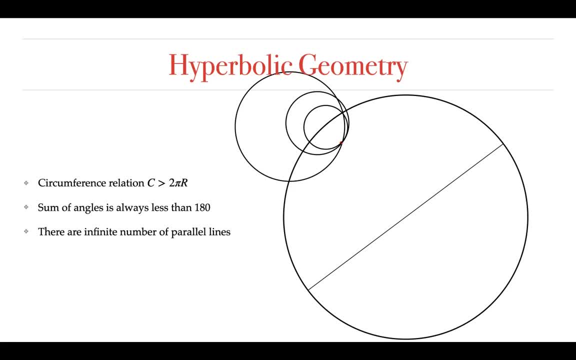 no, i'm not able to recall the exact experiment, but but this is how it was like. so, uh, so eratosthenes is a is a was a greek mathematician, so so so you have two different places, and at one on on some day. 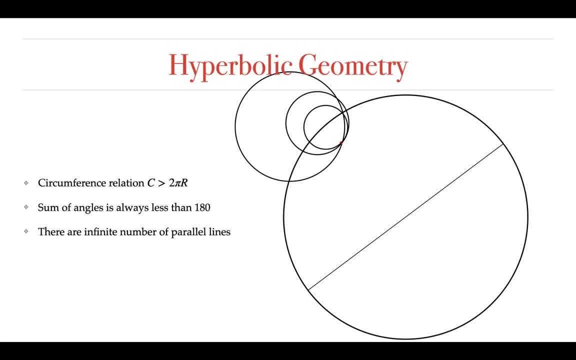 the, the, the shadow of the sun, or or rather the, the sunlight of the sun, should fall, uh, directly to, to the, to the wall, but it does not happen all the time. so, yeah, i mean um, or or maybe not in, uh, so, so, okay, how to say that? okay, um, so, because if it is along, 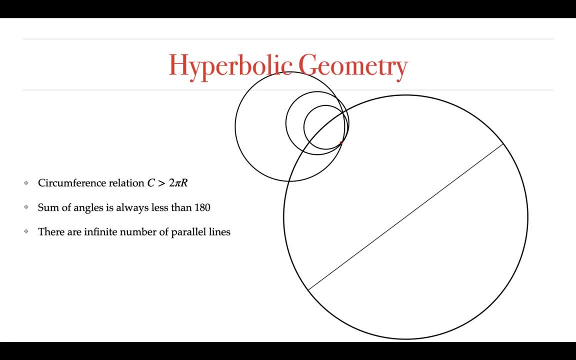 the radius. if it is along the radial direction, then only you can see sun's reflection on the water of the well. but, but, so but, but, if you, if you, according to the raman niyam 123, will be isu 45 grams. But if the surface of the earth was flat all over, you would have seen it in all the wells. 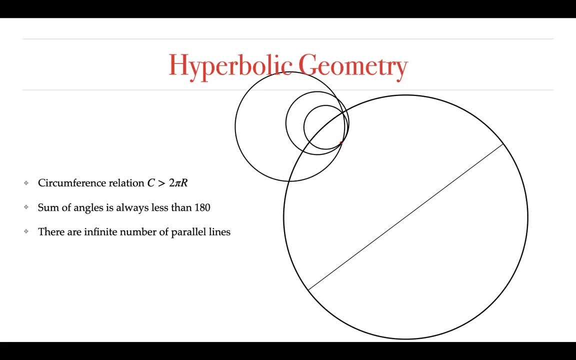 Yeah, Kind of kind of kind of Yes, yes, yes, I understood. So yeah, that's a sort of projection of the sphere on the Euclidean planet, like a circle They used to see. No, whatever you are saying, I am just telling that. 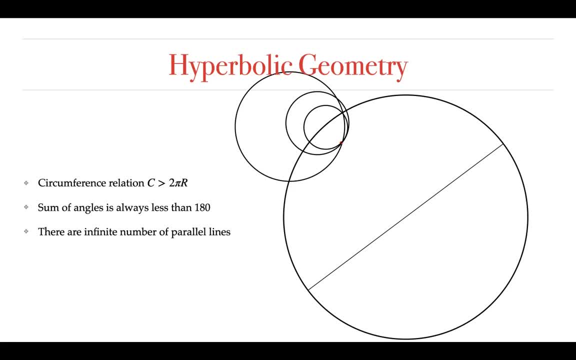 In fact, by using this method, probably Raman has calculated the speed of light also by using similar sort of argument: Okay, Maybe, Yeah, because he used to actually investigate the Jupiter eclipse, polar eclipse in Jupiter, something like that. So by using that only, he used four modes of the Jupiter to calculate the speed of light for the past time. 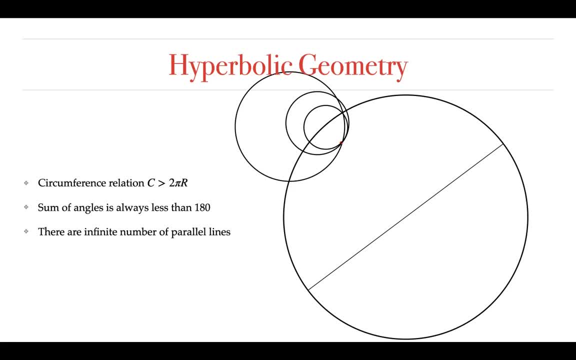 Okay, Oh, yeah, yeah, I have heard about it. That was a very good experiment. Yeah, yeah, yeah, Like this. He also drew geometry on the flat land- only sand only, And he made it put in the sunstone- four stones around the sun- and he did calculate. 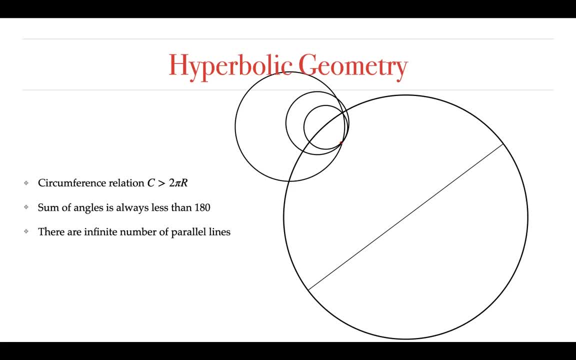 with an incredible accuracy As far as that time technology is concerned. Okay, So, since I am talking about it, so let's say: here is the sun, And if this, and so here, if there is a well, you will see the shadow of the well. sorry, 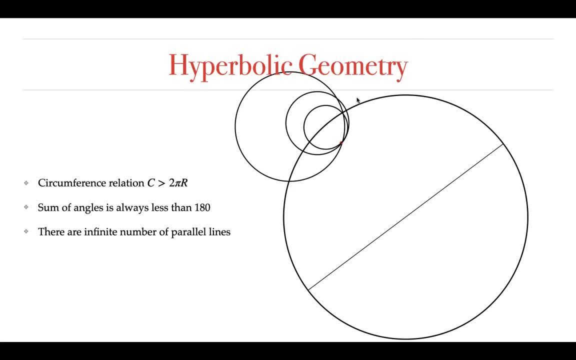 shadow of the well. You will see the shadow of the sun in this well, but you will also see the shadow here if the surface was flat. But since this is correct, you will see the shadow or the sun reflection here, but not here. 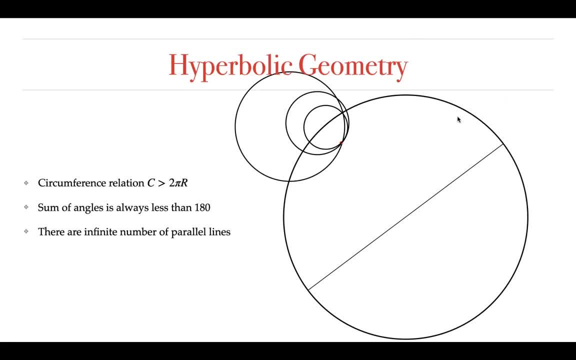 Right, right, right, So. yeah. So the argument was something like this. I mean, perhaps this is not exactly what he said, but he also calculated the radius of the earth using this. But another thing, another thing: How do you mean the black surface? 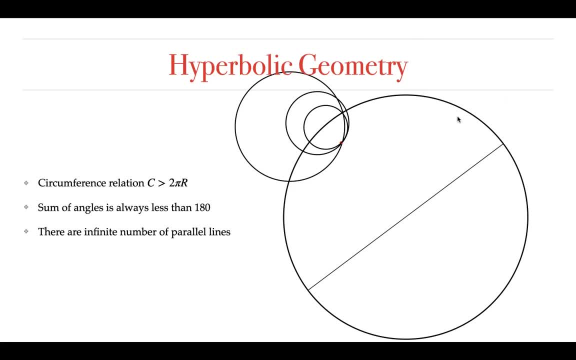 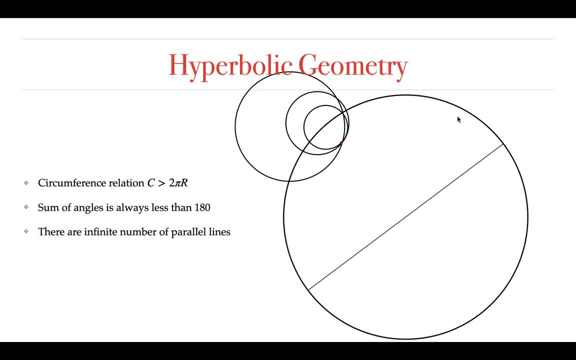 So R is equal to R, So R is equal to R. Yes, Or basically, if there is a wish, then you can get even this kind of thing like this in a plane. then it could've got a plane kind of thing, right. 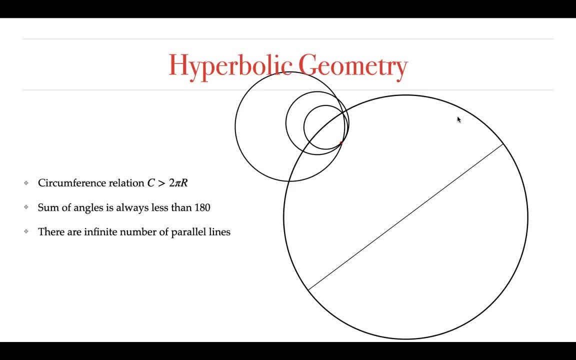 So rectangle, something like that Or something like that, OK, But while you observe the shadow of the earth, it is right there. sorry, it is warm, I mean. so Let's suppose I have a rectangular- plane or a parallel plane. 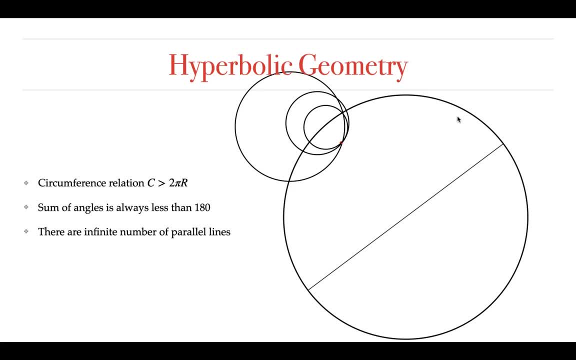 So if I actually clear the shadow by starting a light on it, what kind of shadow I will get? I will get the flat image right. Ok, You will see, keeps changing that okay, but uh, when our shadow, we can feel we are actually seeing it in spirically nature. 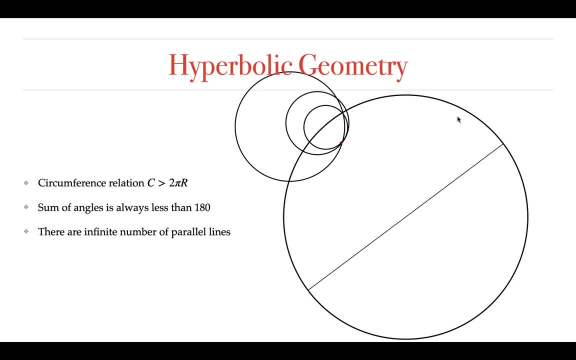 so though, it is just a projection of 3d onto 2d, but it is critical. sorry so, there was a bit of noise in the background so i could not understand what you said, so i'm sorry. could you please say that again? yeah, yeah, here, whatever. 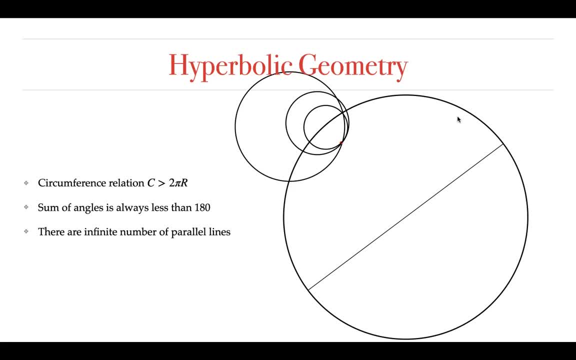 that is correct, uh. but let's suppose imagine there is a flat plane or any sort of wood flat actually. flat plane, okay, flat plane, okay, okay. so what sort of shadow one can expect? it's a flat image, only flat shadow of sun or or what of what. what object: sun. 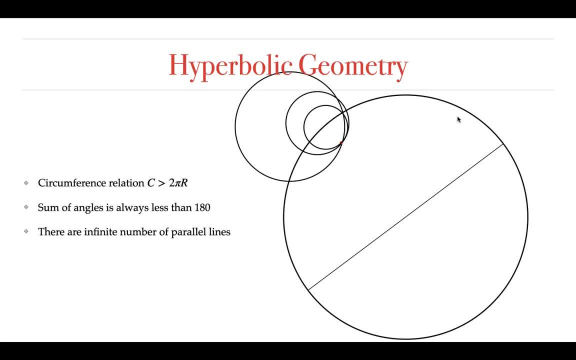 no, no, okay, oh, flat object on moon. then you are. are you saying you you will watch lunar eclipses or solar eclipses? oh sorry, i'm sorry. lunar eclipses, yeah, okay, so, but this is not the case, because that is also another confirmation. how did you not flat? but that was not actually true, because 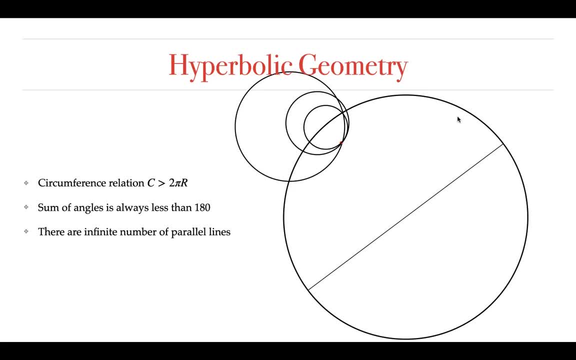 at that point of time, they had some different notions of eclipses. i see, i see, oh they, why then copernicus? copernicus still was not in the time. okay, yeah, i mean, at least in indian concept they would say that there are demons, rahu and ketu. they are believing in geocentric 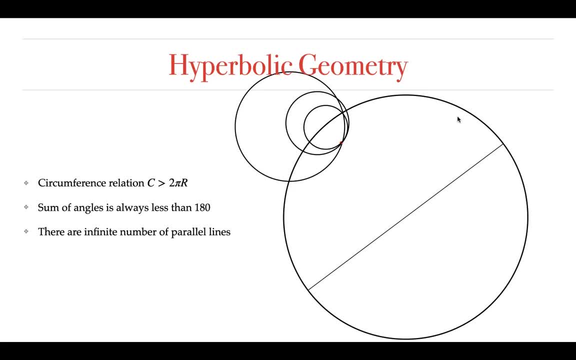 right, it's not just that, not just that, but. but i don't, but i'm not sure, i'm not sure whether they had the right or whether they had the right notion of what eclipses are or what, what cause eclipses. i mean, you don't have to have the clicker type of flow system, and for that matter. but 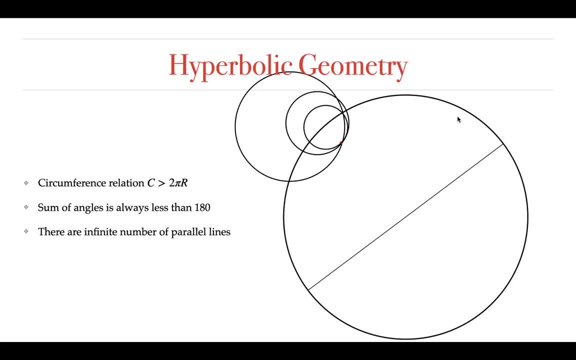 you have. but you should have because we are seeing, let's say, solar eclipses. for solar eclipses, you just have to understand moon, earth and the sun system- and for the and and also for the lunar eclipse. but i'm not so sure whether they knew the mechanism like: how is this happening? 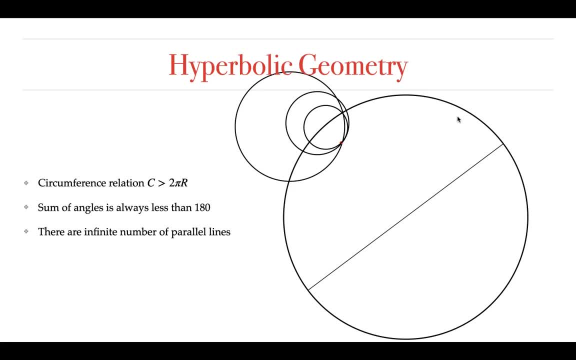 how is that happening? because, it is understood, did not know it, because if they didn't resolve the solar system arrangement, uh, i'm not so sure about that that they that actually knew it because, uh, so perhaps, maybe, maybe after renaissance, let's say in the 15th or 14th century europe. 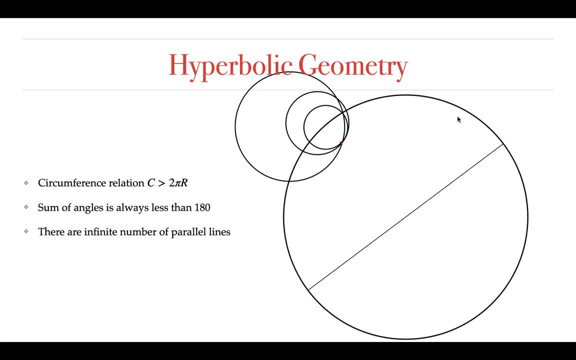 only they knew about the mechanism, but i'm not so sure. i have to check it. so, yeah, so based on that, so given that the mechanism is not clear, you won't be able to um, what attribute? the circular image or on the on the moon? uh, one thing i want to ask, so 1610. 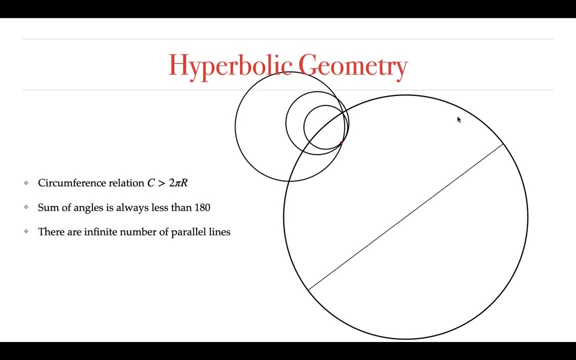 ah, if i can remember correctly, 1610, i think, uh, here on which geoffrey discovered his salnau. okay, capitalist, okay, so i'm not saying some kind ofulturistic problems. i mean, you know, same with solar eclipse, but the science of solar eclipse has not been proved. now, so as to how much solar eclipse? 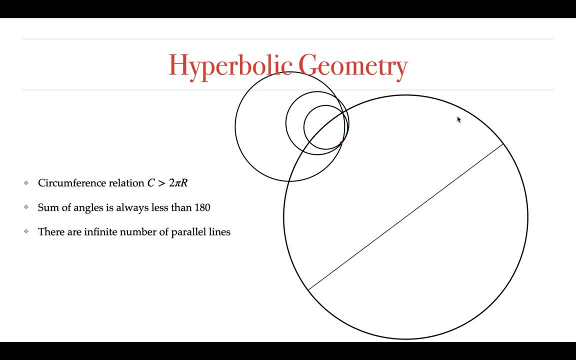 will have now. uh, speak to me again in the last few years like: why does this century something very exact here, but then earlier we were talking about BCs, So at least this was this should. so when I am saying that this idea was not clear, I am really talking. 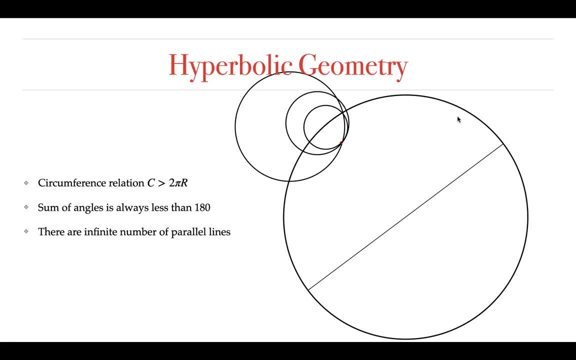 about BCs before, let's say some 200 BC or maybe 100, 180, 280.. Certainly not, certainly during, not that, certainly not during that. I think they must be not be knowing the exact mechanism, there might be some speculation. 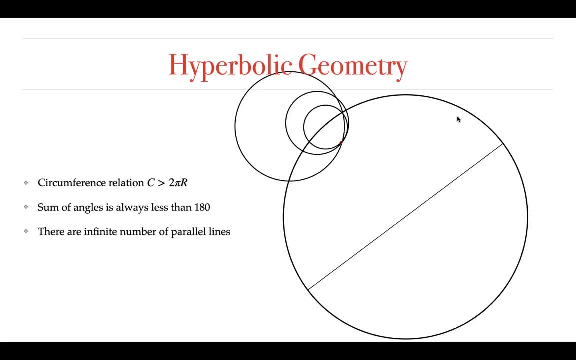 also, Solar system was clearly designed only after Kepler came into picture. is it not What celestial mechanics has taught us? No, that is true, but then it has nothing to do with the solar system. in my opinion- I mean it- it has to do with the fact that 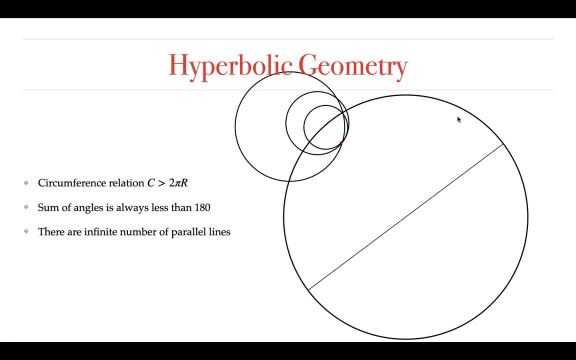 first of all, the shape of the Earth is spherical and somehow earth comes in between moon and sun, or moon comes into the sun. No man, I was wondering because, sitting in a small witness, it was now sad we are talking about the PSA today. Paragruha, that consciousness has entered into the world. healthcare: 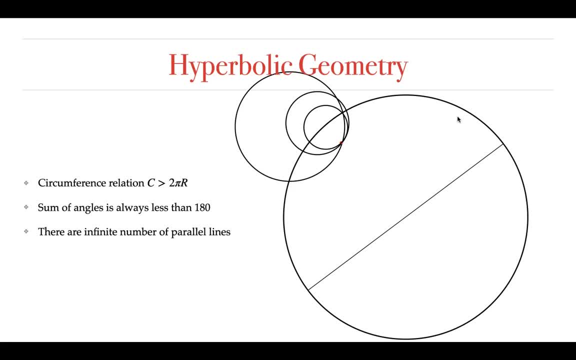 here. right Answer is to come and go back to it. it is the same information, but是這樣. competence between sun in the earth. so that's how eclipses happen. yeah, yeah. but if they would have to actually skip those mechanisms by saying somehow it would have happened, maybe they would have some. 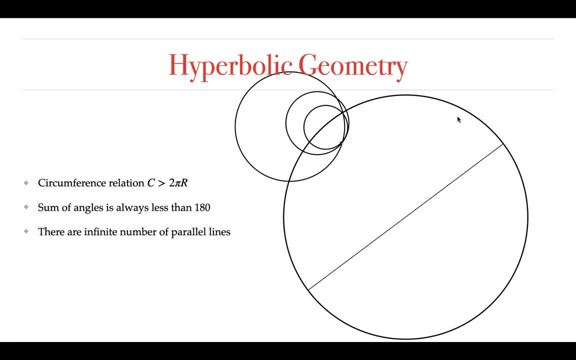 uh vague idea of how the thing is going on. but what i am saying? the exact quantification or the perfect repeatability of the data, or prediction uh had occurred after the prediction of the plus laws- i think that's what the historian says- or maybe after the discovery of newton law, of 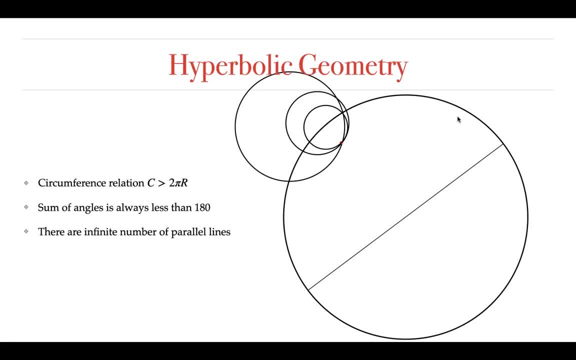 gravitation. yeah, that explained the mechanism. that explained the mechanism. but the proper arrangement of the heavenly bodies actually somehow got finalized after the toponikos theory came into picture and followed by kepler and dichro, all those things. okay, maybe it's a lot of historical. 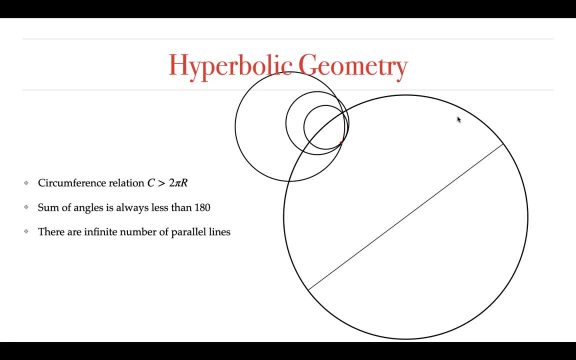 debate. i mean so. so this is what i can think of, because it was perhaps not worth the effort. why would you make 20 kilometers long, 30 kilometers long, just to know what is the geometry of the? there are some more important questions to be answered, at least mostly. 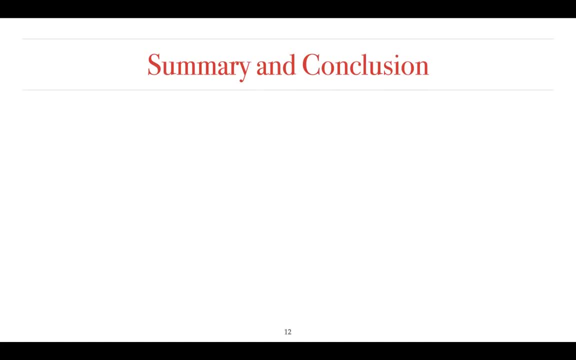 money making and rule the one: uh, maybe not even that, not even that, but then perhaps there are, there are other important issues, so it totally depends. so if, if, um, so we really pursue those things which we feel are important, exactly, this is the most precious statement, this is the most important statement. 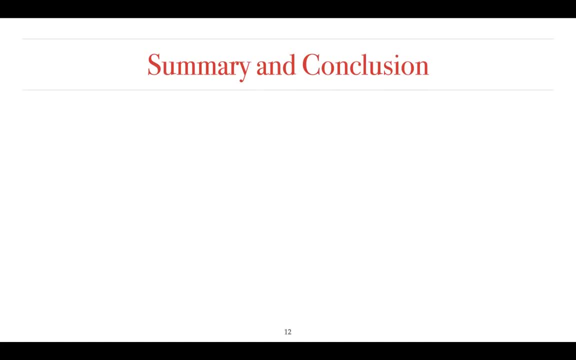 the most precious statement. ultimately, this is the statement which decides the destiny of any social society in a given time. that is true, i mean so, so, because this is the statement. i mean so, uh, i mean so, so, so. perhaps this is not related to this talk, then, but, but, but uh the uh. aristotle had his 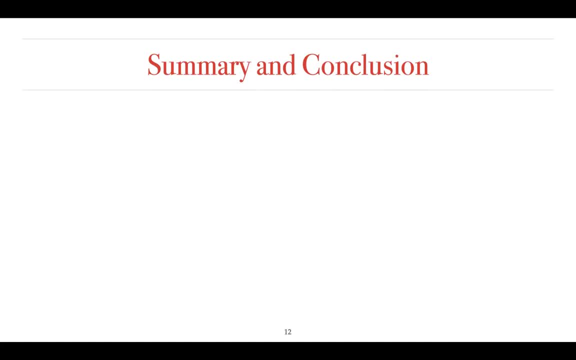 had his- uh what? the, the school of logic. there were also stoicism, and, and there were so many schools of thought and at that time, because perhaps society needed them, and and, and that's why, and that's why they were invented, we, we also had some aristotelian laws of motion. i mean maybe 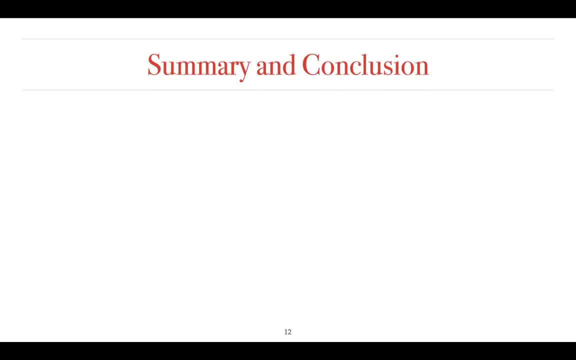 he was just curious to know why, uh, why motion happens, or or can we quantify motion and so on? but but it depends whether it's whether you feel it, you, whether it is useful or not. uh, if you don't. and important, you will not pursue it. i i'll just, uh uh, ask you my question because the day before 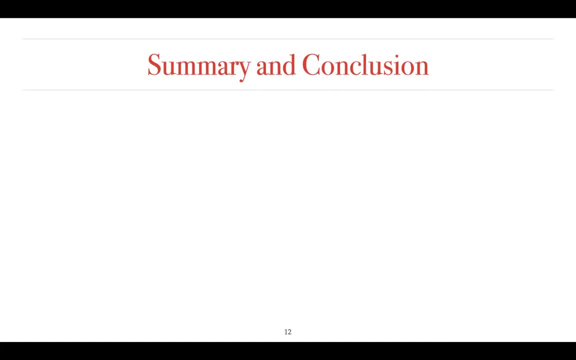 yesterday in iop- uh, i have i had a discussion with one. so in in those days, the days that we were talking about aristotle and all those natural failures, of course, personal scientists, so those people used to believe actually things moves for some, for some time and then uh stops because uh body gets tired. okay, kind of. so he, this is how the history. 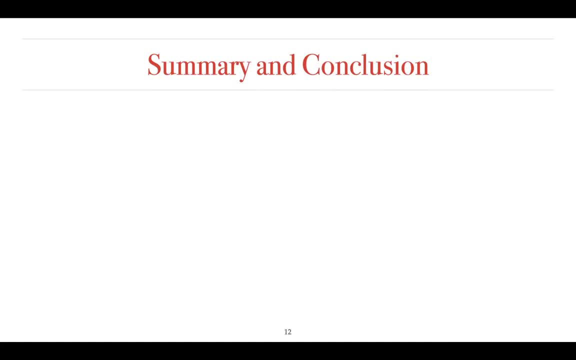 of promotion began, uh, and now also we are saying system actually always try to minimize its energy so that it will remain in a much stable state. so it is not the same thing, but in a different style. i mean and and also the gravity theory. i'm asking, i just want to know your. 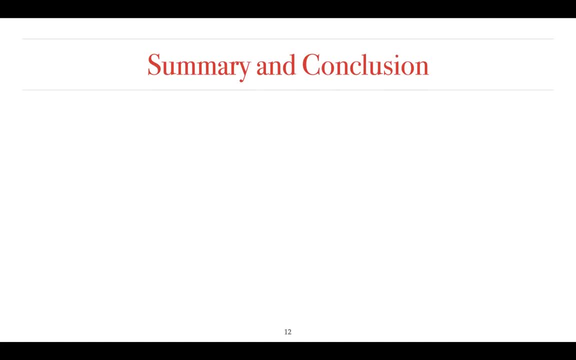 i think i also have heard about that. uh, so what was the name of the book? so, so there is one book which was forwarded by ed witton- um, okay, yeah, that was forwarded by him, though not written by him but forwarded by him. um, i'm not able to. 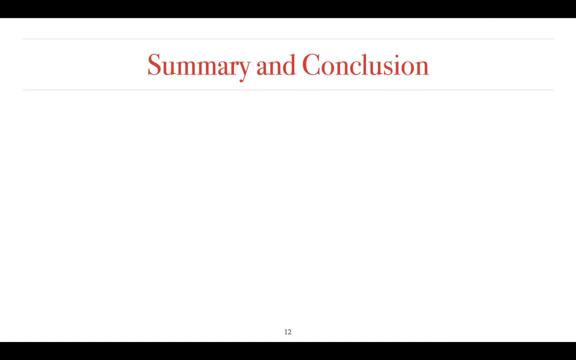 call the name of the book, but i think in that book a lot of history is covered, so so so one part that i'm sure about is that that aristotle used to believe that. um, so why? okay? so why would object fall downward? because, because it will, there's a kind of bond between earth and that. 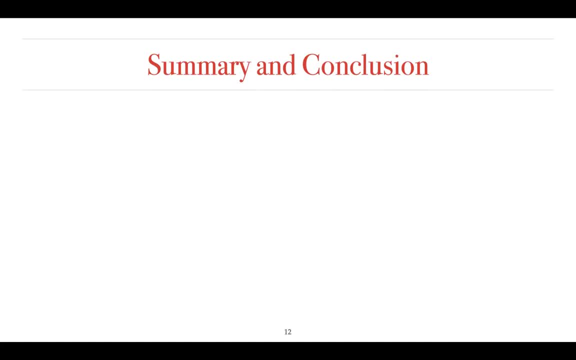 object and why it accelerates. because as it is falling and it is going toward the center of the earth, it is becoming more and more excited, more and more, and thrilled, something of that sort. so that's like that, like that, yeah, yeah, like that. only he, he mentioned this statement instead. now. 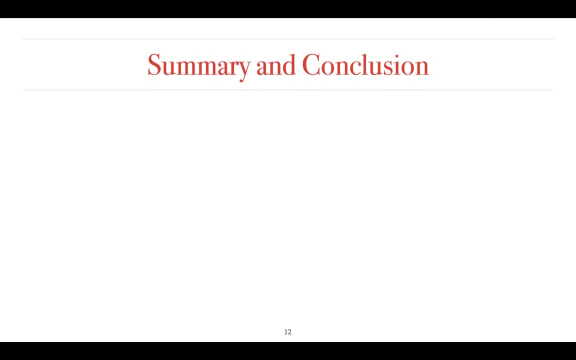 we are saying: every system try to minimize its energy and to remain, to remain in the stable configuration or system. yeah, straight up, and i think so. that is what they have told two thousand years before somebody tried to take rest. that is that is why he doesn't move always. 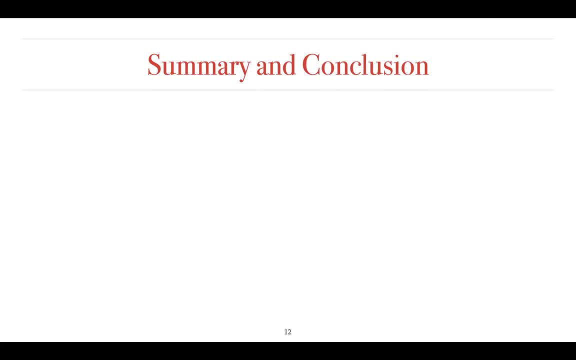 uniformly or try to keep on moving. yeah, sure, so, okay, so, okay, yeah, so so. so what will we discuss today with the case of uh 2d surfaces? i mean, if you go to, if you want to go to 3d, these will be quite, i mean. 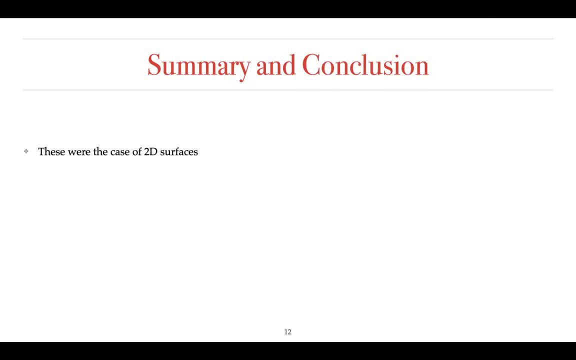 perhaps very, very difficult to imagine. so, but then 2d would, uh, give um example or the feeling that how would that what we would do in case of 3d? so so there is one more technique, which is called parallel transfer, which we have not discussed about today, and this is also also useful to tell. 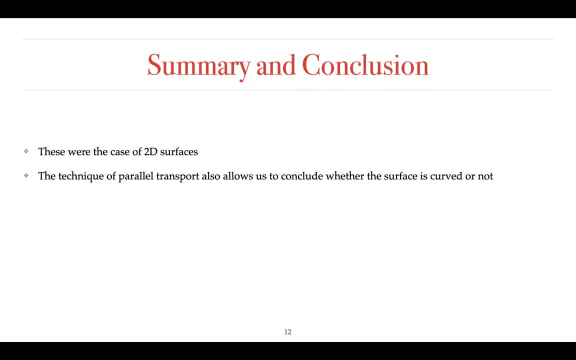 you whether the space in which you are in this curved or not. so curve, curved is, we say something if some space is curved, if it does not follow the rules or the axioms of the euclidean geometry, but but in in whatever case, whatever case you take, if you take very small region, 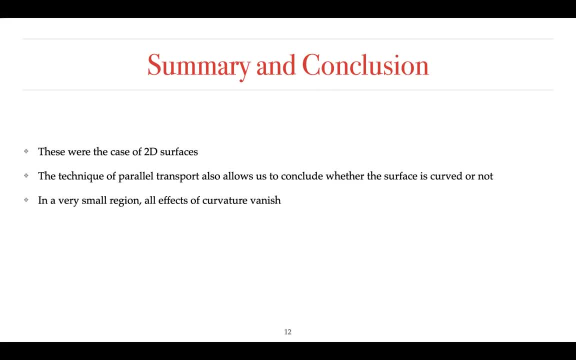 so. so here i should have put very important, because so the the smaller the region, the the more it will approach towards the euclidean case. so so, if you recall the example of the sphere on the surface of sorry, if you recall the example of triangle on the surface of the sphere, 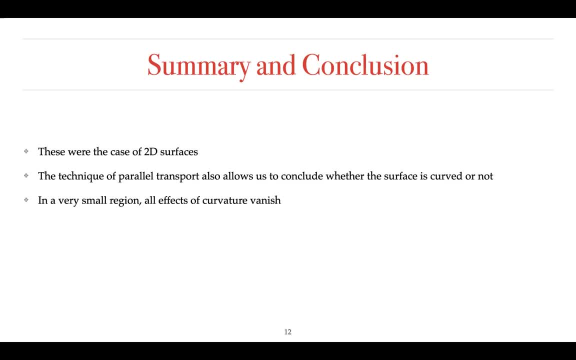 if you just shrink the size of the triangle, the sum of the triangles will approach to 180 degrees, as you can check. i mean, of course, you can check it on the surface of the earth. because how? because we cannot make so, uh, so large triangles. so because the surface of the earth can be. 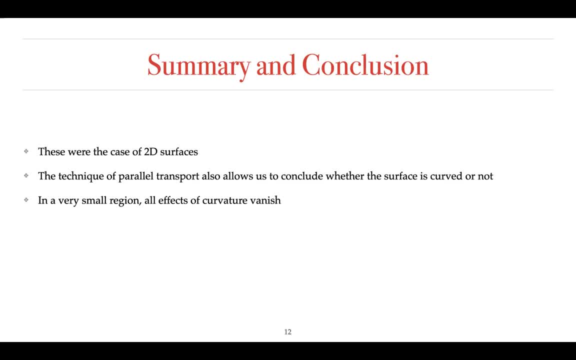 very well approximated in in a very small region, as the, as the plane. so whatever triangle you draw, you will always get some of its triangle equal to 180 degrees. so, so, so, so, this idea, so, uh, the idea of a manifold, which we have also not talked about today, 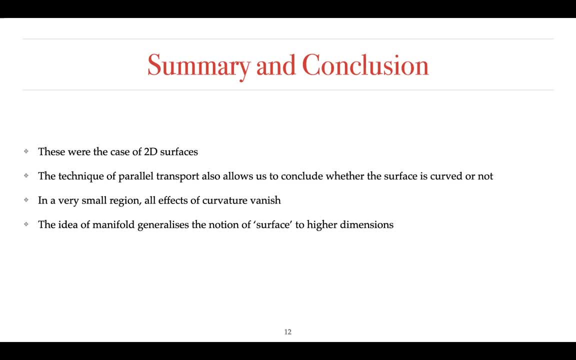 generalizes the notion of surfaces to higher dimensions, because manifolds are some kind of mathematical objects which look, which locally look like flat spaces, when you, when you talk about very small regions, i mean of course these have precise mathematical meanings and these perhaps can be talked about in in future talks, so so, so then this i mean so, uh, in this context, the general 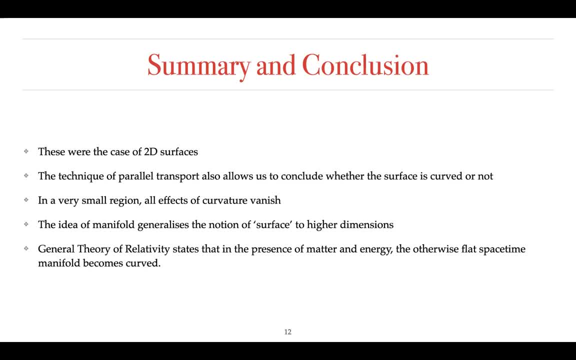 theory of relativity it states that the in the presence of matter and energy. so so i've talked about the manifold, the space time. so here we use the notion of a space time manifold. so in in the presence of matter and energy, the space time manifolds become curved. 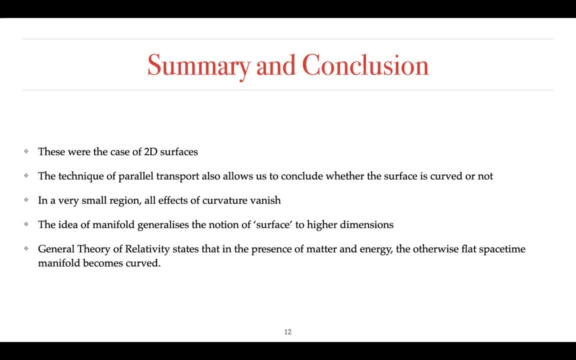 so, yeah, maybe we will talk more about general relativity itself. so, um, uh, so, and i will also try to reduce the number of equations in it, because that is also true if you don't really use math in it at it is my opinion, if you are studying general relativity, then perhaps you 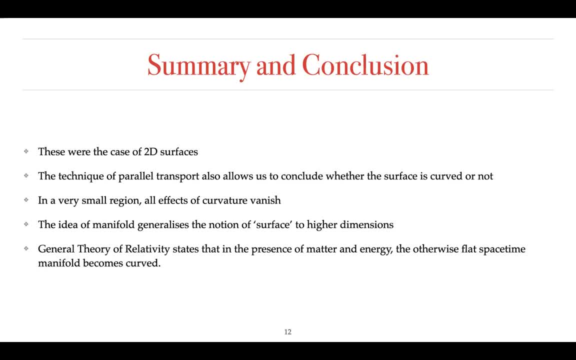 won't understand or you won't take anything out of it. i mean these. so some math is kind of inevitable in it. so you have to introduce kind of tensor or but you have to introduce but but when you? but when you talk about the equivalence principle etc. equivalence of um, like 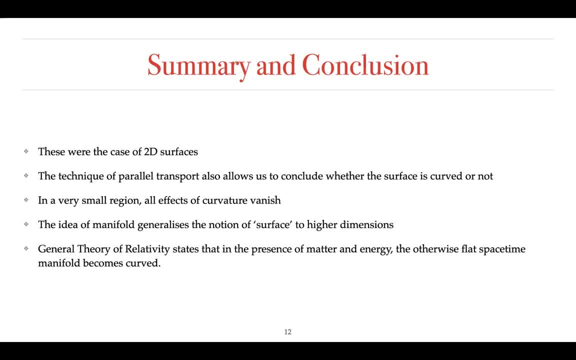 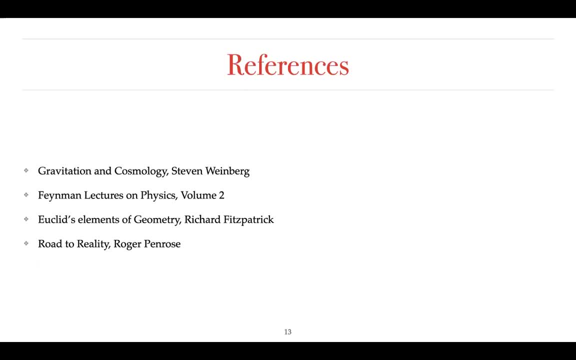 constant acceleration and gravitational fields, then that's a different story, but then, if you were to get some numbers out, math is inevitable. okay, so these are the references i use for this. so, um, i mean, this book is really very good to read, so if you find time, you should definitely. 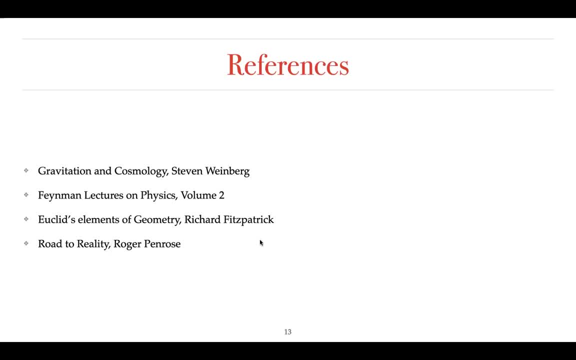 read this book. oh my god, it's really. i haven't finished and i'm like: no, no, not. i mean i i just said about 15, 20, 3 chapters, not more than that. oh my God, how many it's. the philosophical content? it's 30, 40.. no, no, it's in more, it's more than that. 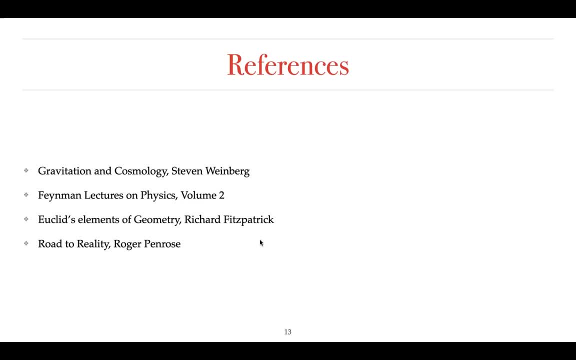 i think approximately 40 or anyway, so. so then i shouldn't have about 20, 30.. so maybe i i get only 5 or 10.. okay, this is exceptional, so i i think you can discover theMark gebe예요 MP Ch 봐요. I don't remember your name, García Eでした. earlier, when i spokeaten'su'realaba alves Carlito" troviagvoi i этиobag anymore. " Why was it boy". Doris Marmaris stone, heewooh.